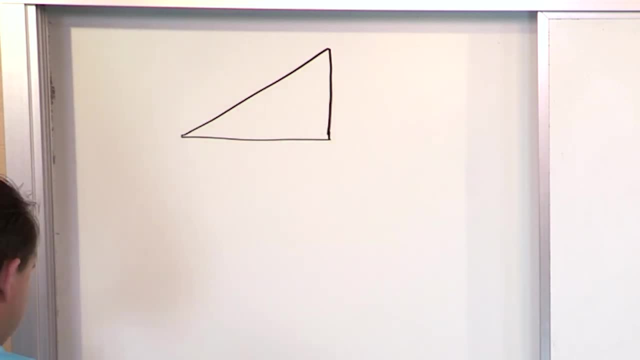 You talk about triangles all the time in trigonometry. That's what it's all about. So you have some kind of triangle and this is a right angle, which means it's 90 degrees over in the corner And there's some angle. 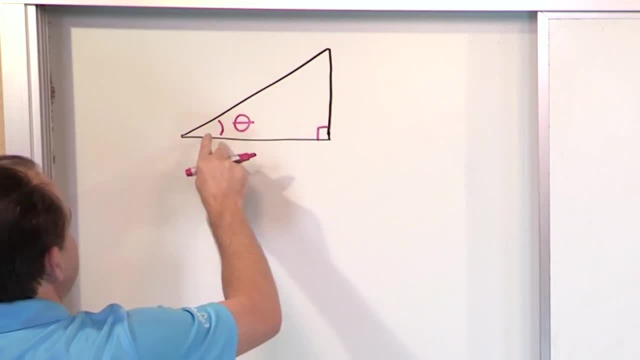 Like I told you, you might have a wedge. A lot of times in physics problems we have a wedge and we call this angle Theta. So theta, don't let it scare you. It's just another variable, like X or Y. 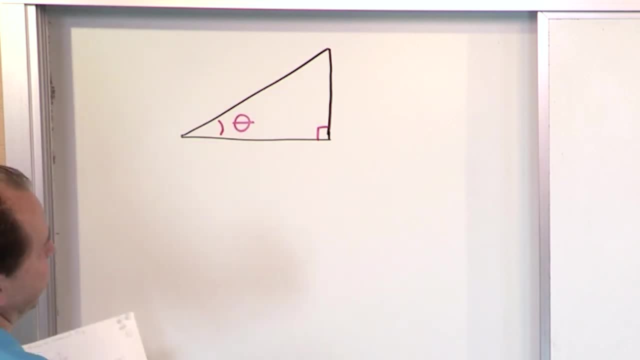 This could be 15 degree angle, or this could be a 35 degree angle, or a 70 degree angle, or whatever. Of course, as the angle increases, the the steepness of this wedge, you know, gets taller, or whatever, But this is a general diagram here. 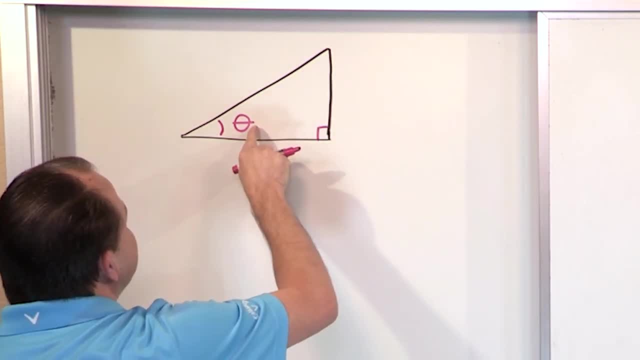 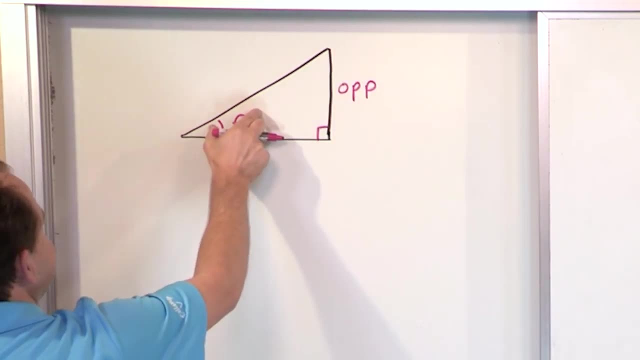 Now we label the different parts of this triangle, We say that relative to this angle, the opposite side of this guy, we're going to label it opposite. OPP for opposite. and relative to this angle, this side right here is adjacent. A, D, J, We call that adjacent. 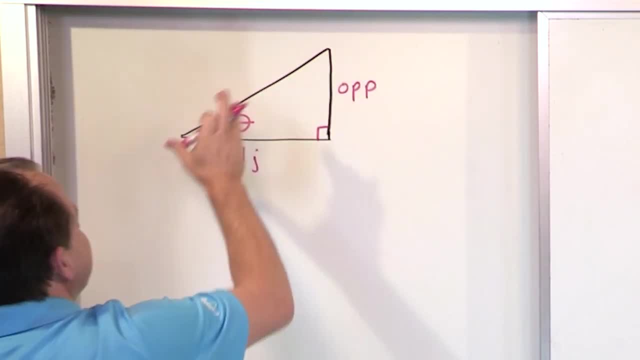 So adjacent means the side kind of close to the angle, Opposite means the side opposite the angle. And then the very longest side of every right triangle is called the hypotenuse. And I know that you all know that from basic, from basic math. 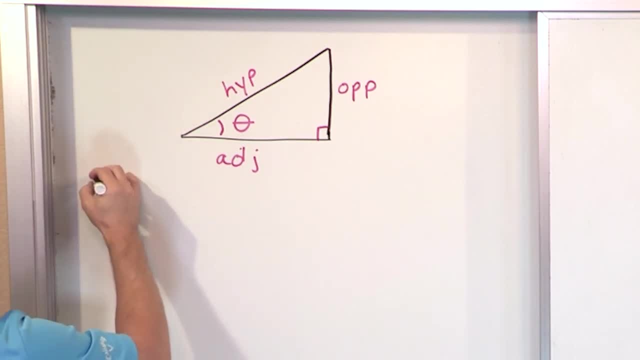 Now also in basic math, you learn something called the Pythagorean theorem. Don't forget Pythagorean theorem. Don't forget that with right triangles like this, you always have the Pythagorean theorem at your disposal. The physics problem will never say: use a Pythagorean theorem to solve it. 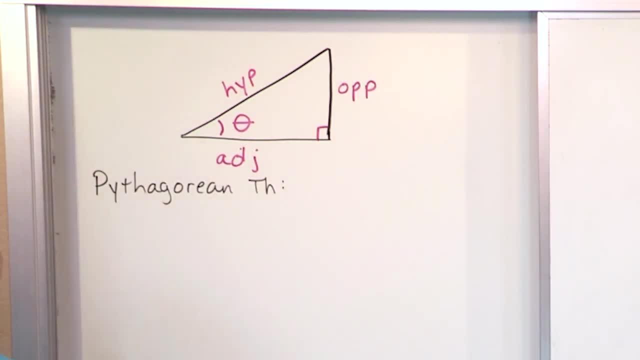 It'll never tell you that. You just have to know that you can use this for every right triangle Pythagorean theorem. If the way you learn it in geometry is, C squared is equal to A squared plus B squared. In this equation, C is always the hypotenuse. 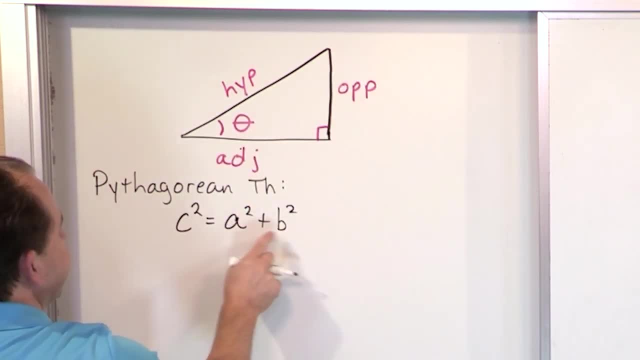 It's always the longest side of this triangle. The other two, since they're added together, really doesn't matter The adjacent or opposite doesn't matter what you label them. So the way you Read this in terms of this triangle that we have right here, 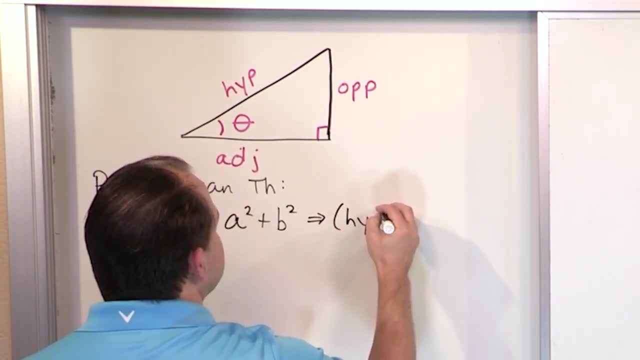 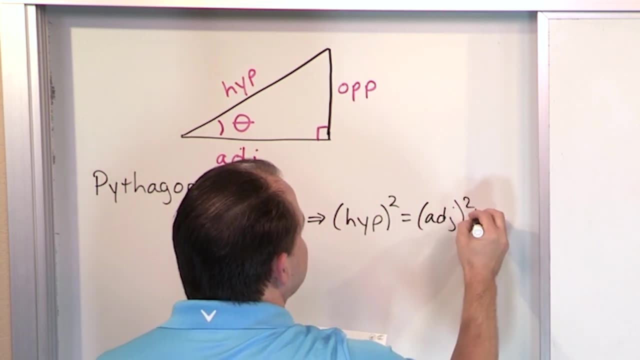 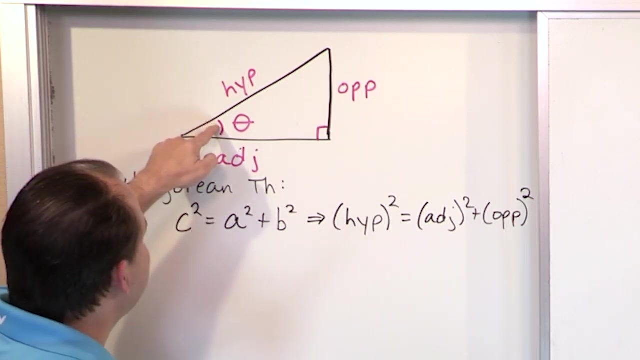 Since C is the hypotenuse, we'll write it as hypotenuse. squared is equal to- And again, I told you it really didn't matter, So we'll just call it adjacent squared plus opposite. What does this equation mean? That means for any right triangle, no matter what the angle. here is: 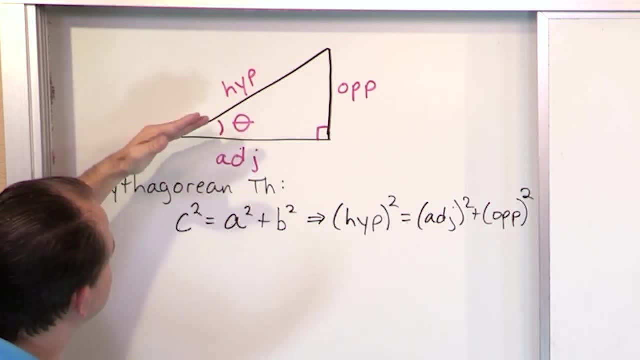 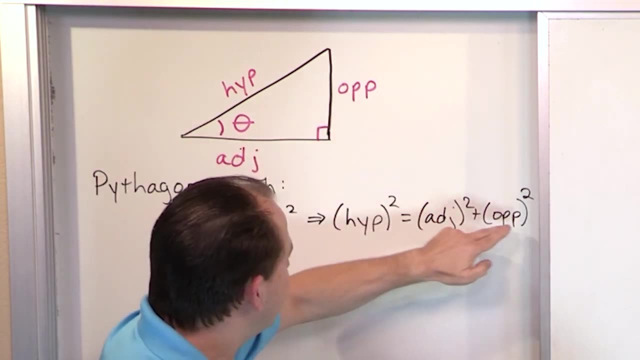 whether it's 15 degrees, 30 degrees, seven degrees, really slender triangle, whatever, Doesn't matter. if you know the length of the hypotenuse and you square it. And you know the length of this and this and you square them separately. 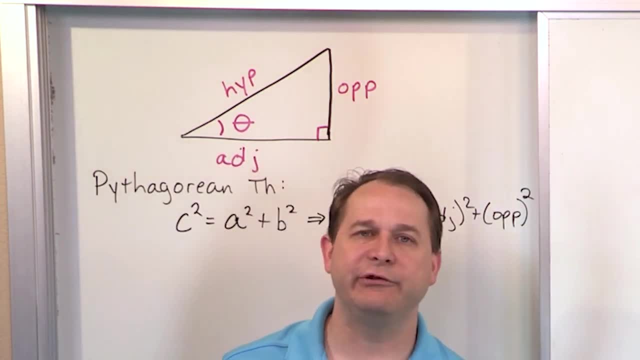 And then you add these together, They will equal each other always. So it allows you to find the third side of the triangle. Okay, The reason I'm bringing this up is because we're going to use it a little bit later, But it's important for you to know that it applies to all triangles, not all triangles. 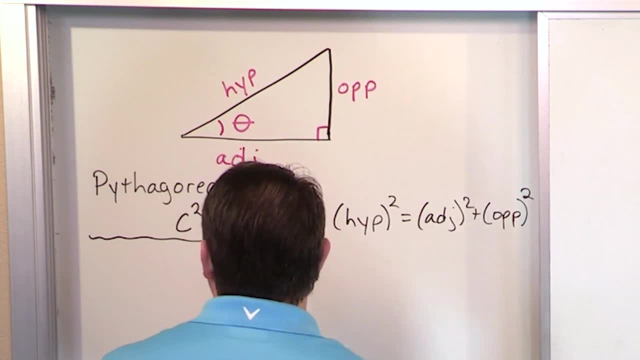 All right. triangles with a 90 degree angle, like this one here, All right. The next thing we're going to do, we're going to talk about the fundamental trig functions. Now, In truth, there are more trig functions than the ones we're going to list here. 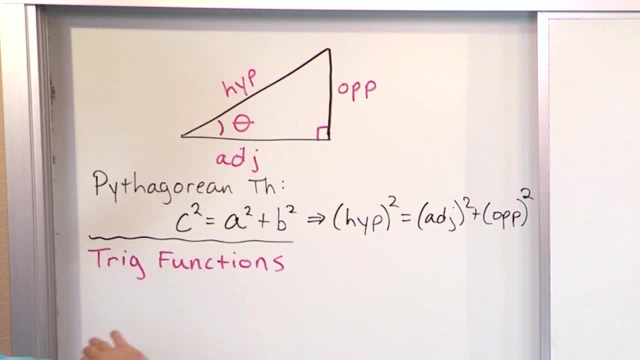 But these are the trig functions that are most used in physics. We come across anything more complicated than this. I'll explain it as we go. The first one I know that you all heard of It's the sine of some angle theta. Now, in a real problem, you'll put a number here like 45 degrees or something. 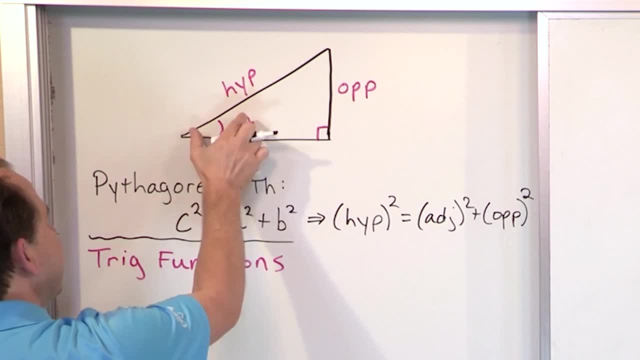 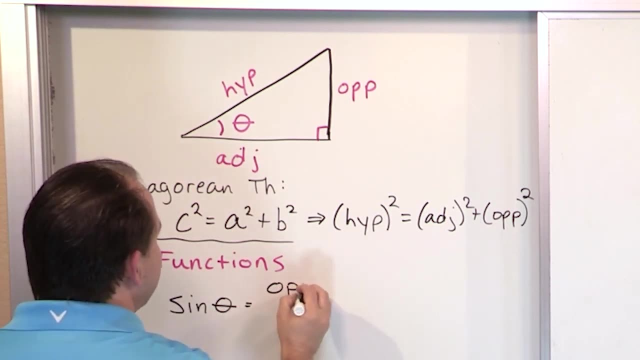 But we're drawing everything generally. So we say the sine of whatever this angle here is is defined to be the opposite side over, divided by the hypotenuse. So you literally take however long The opposite side of the triangle is and you divide it by the hypotenuse, right? 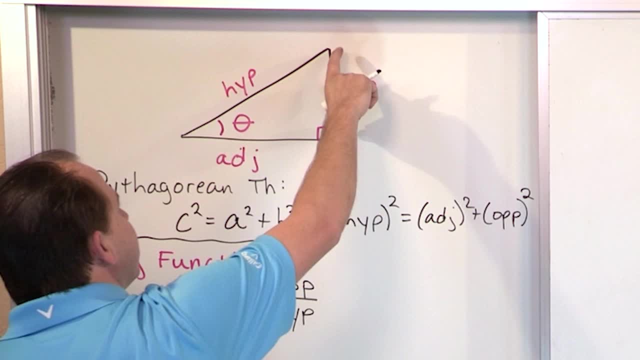 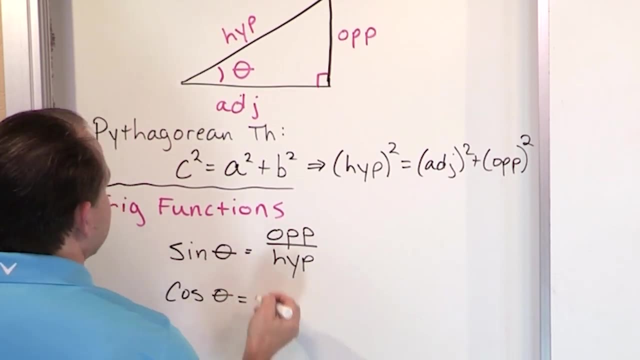 That's defined as the sine of this angle. Notice that the sine of the angle involves the opposite side. Okay, Remember that because that's going to be important. The cosine of the angle of this triangle is equal to the adjacent side, divided by the hypotenuse. 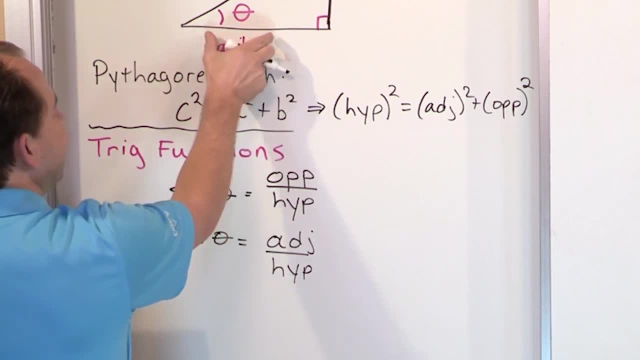 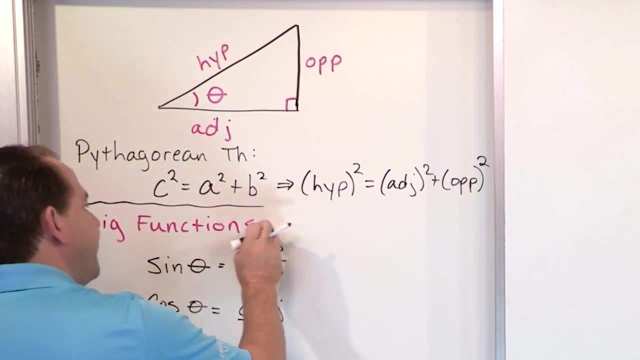 Again, notice that the cosine of the angle involves the adjacent side of the triangle. That's going to be important, So remember that. So just by, without going any further, The sine of this angle involves something to do with the opposite side of the triangle. 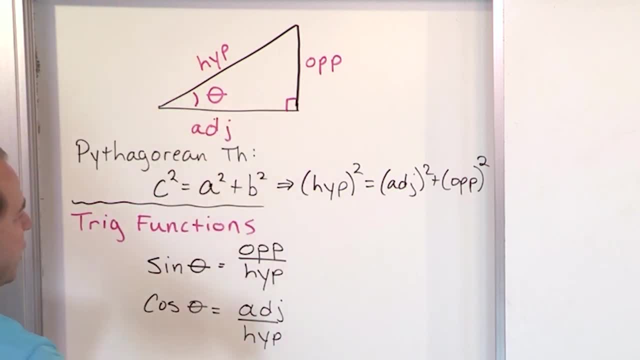 The cosine of the angle has something to do with the adjacent side of the triangle. They both involve the hypotenuse, But that's kind of not so important for right now. Well, it's important but it's not going to be not trying to make you remember that right now. 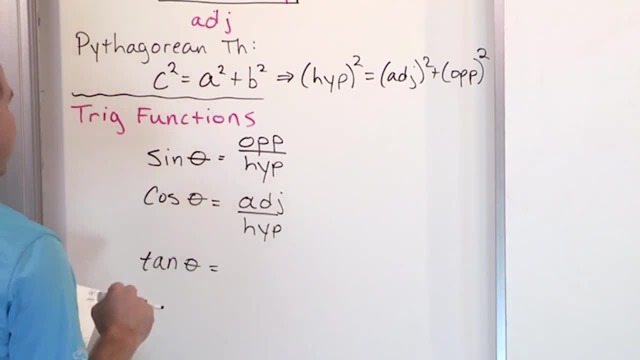 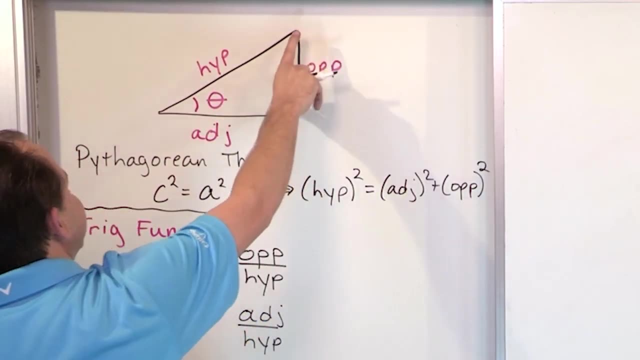 The tangent of the angle, which actually we're not going to use quite as much in physics problems. Most of the time you'll probably use one of these. You'll see why as we solve vector problems. It's defined as the opposite side divided by the adjacent side. 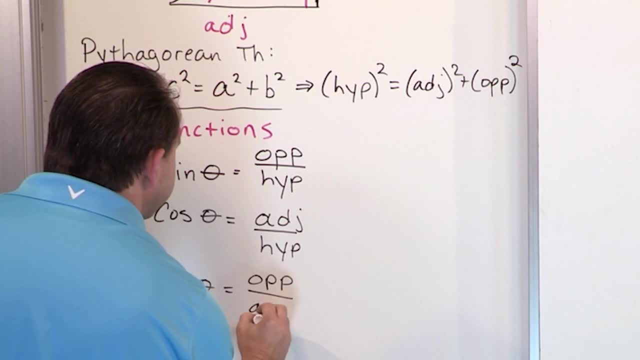 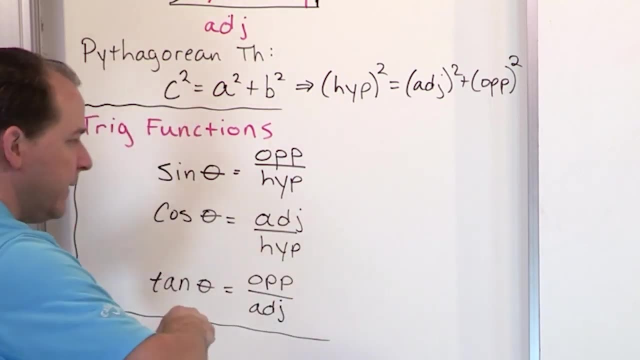 So it's the opposite, divided by the adjacent side. So these are critically important. If there's one thing that I would write down in this review of essential trig, First of all it's called a review. I expect you have seen this before. 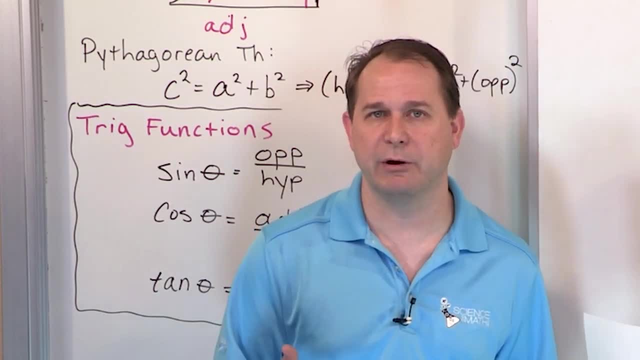 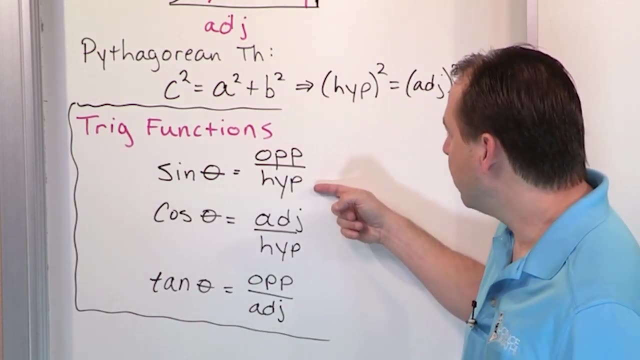 And it's essential trig, which means it's not everything, It's. the most important stuff for these kinds of problems Is, I would want you to know these three things: Sine, cosine, tangent, If that's all you remember, That sine is opposite. 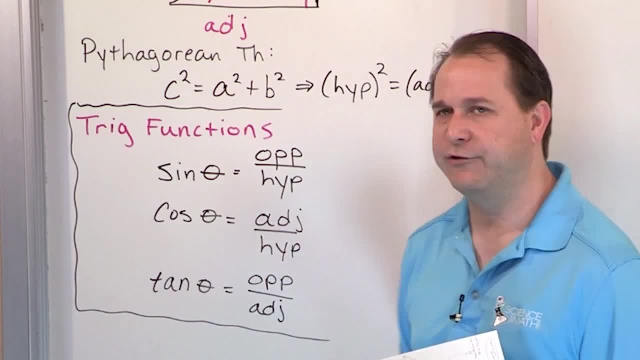 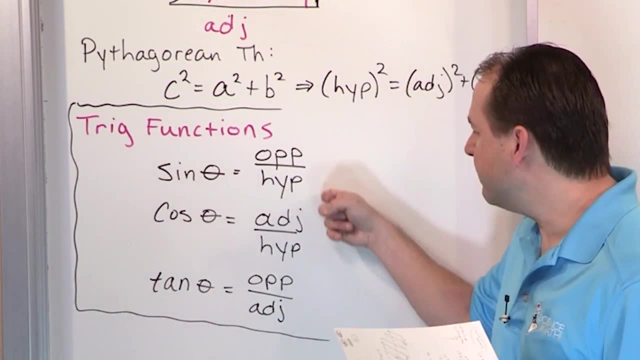 Over hypotenuse. Cosine is adjacent Over hypotenuse, Tangent is opposite Over adjacent. If that's all you remember, then you can solve a great many problems, Because most everything else that I'm going to talk about in this lesson is just going to be messing around with these functions to do useful things. 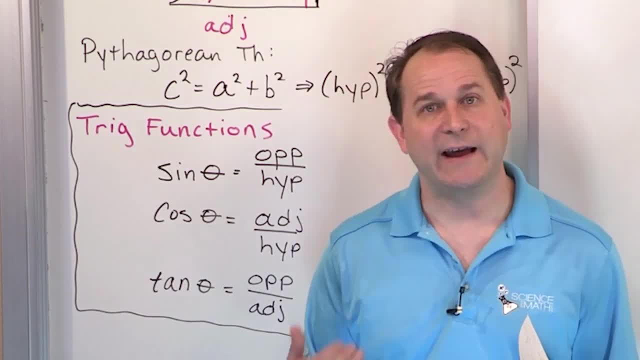 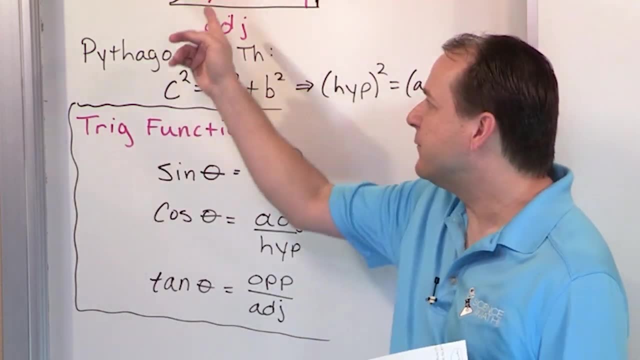 So if you only have to remember one thing, remember these and understand what it means. I know a lot of you looking at this say sine theta. What does that really mean? It's literally just a fraction Sine of whatever this angle is. don't even worry about what the label is. 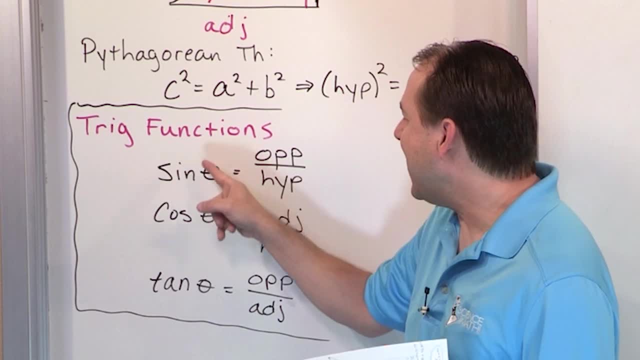 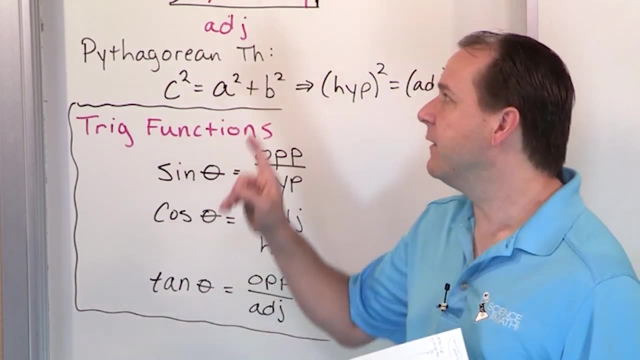 It just means that something that's related to this angle is defined as a fraction, defined on this triangle, And if you forget which is which opposite, adjacent whatever, then just remember how to put this picture together and draw this picture on your test. 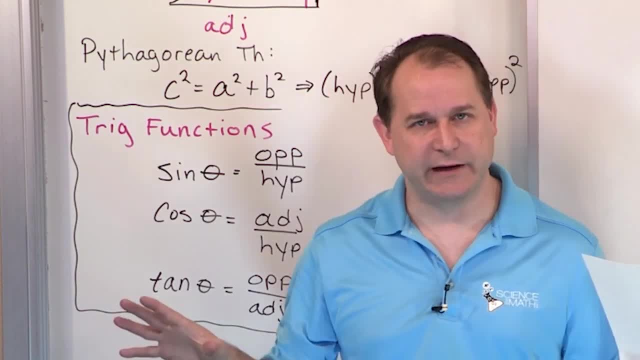 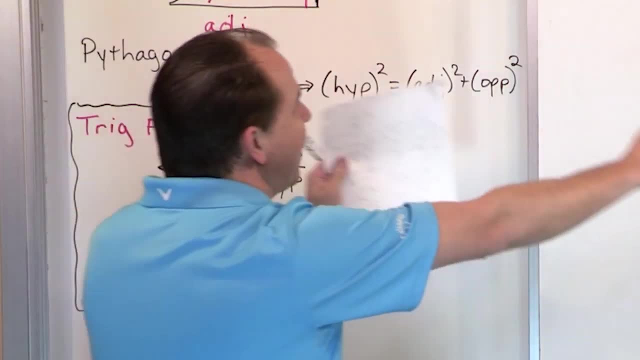 For many years I had to draw right triangles and label everything so that I would keep it straight. Now I just remember it. But if you need to draw that picture, please do draw it Now. we're going to take this and we're going to do something practical with it on the other board here. 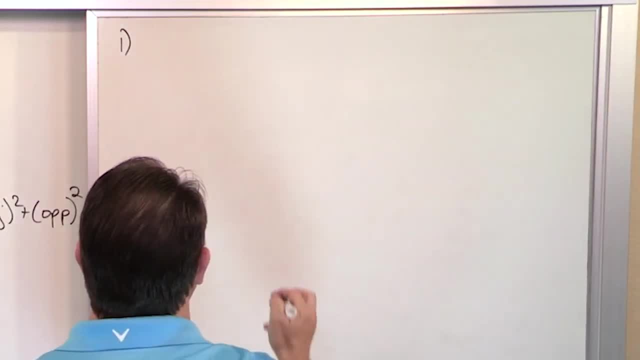 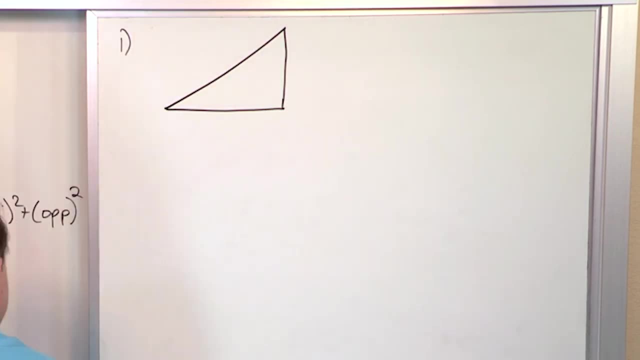 So let's solve a quick little problem. This is not exhaustive. We're just going to do a quick little problem just to illustrate what I'm talking about. Here's a triangle like this. Now, inside this triangle I'm going to again. I do not know what this angle is. 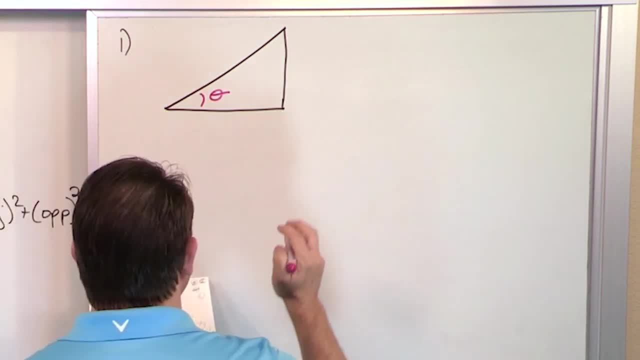 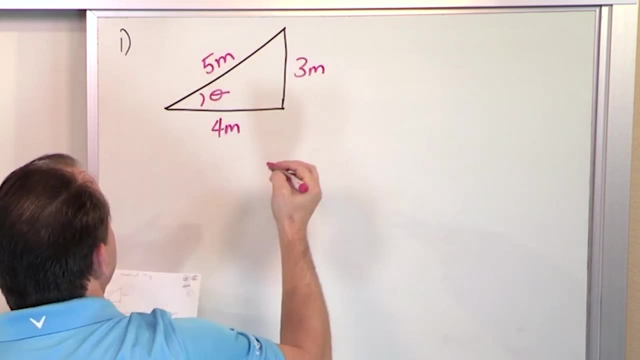 Sometimes I do know what the angle is, but in this case I don't. But what I do know now is that this side is three meters long, this guy is four meters long and this guy is five meters long, And I'm saying this is a right triangle. 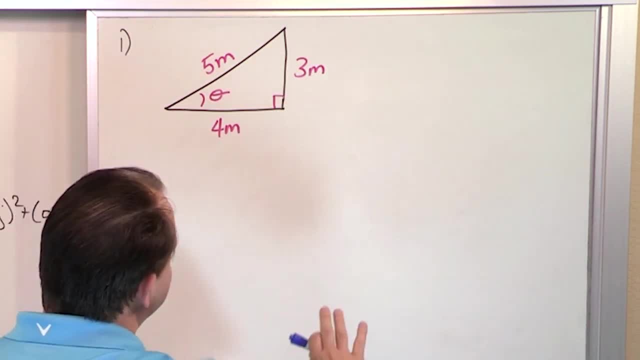 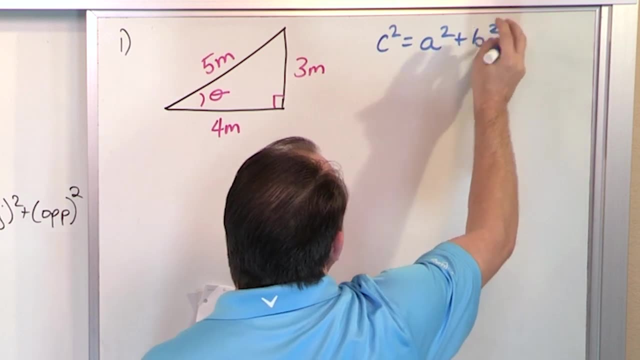 First of all, you can always verify this is a right triangle. You should always make sure this is a right triangle. How? Because we know that C squared is equal to A squared plus B squared. This is true for any triangle that has a 90 degree angle on it. 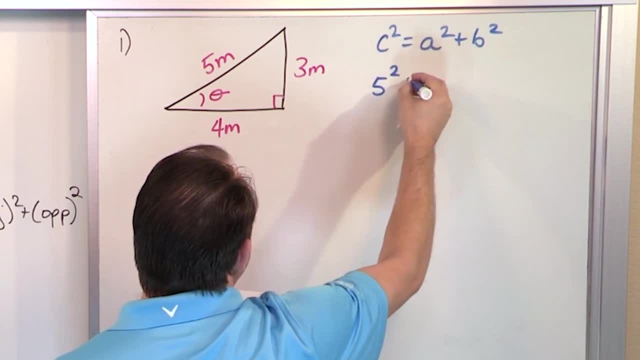 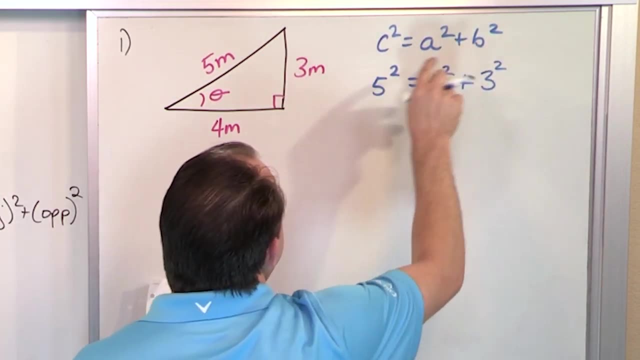 C is the longest side, so that's five. Now we have to square it And we're going to check and see if it's equal to this squared plus this squared. Notice that A and B doesn't really matter because, see, I did four squared plus three squared. 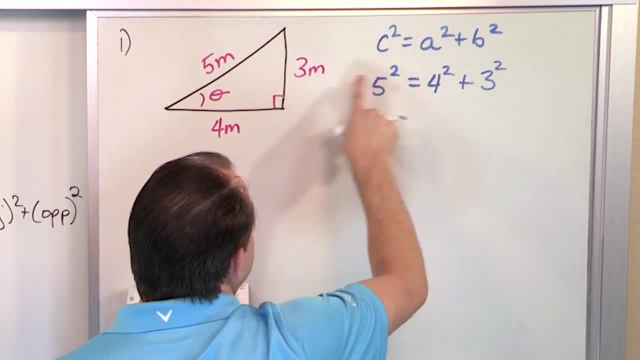 If I called A equal to three instead, then it would still be three squared plus four squared, So the right-hand side would be the same no matter what. So the only one you're going to do is you're going to do this. The only thing you really care about is to make sure the longest side goes in the C column. 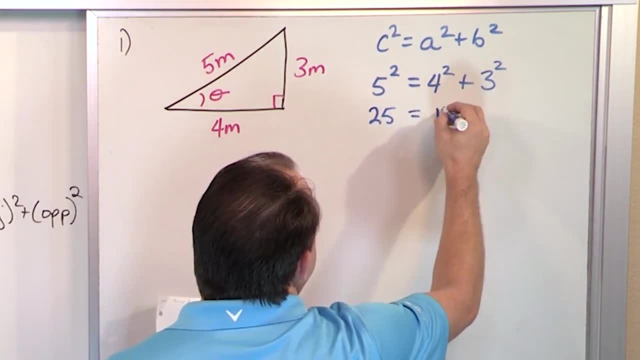 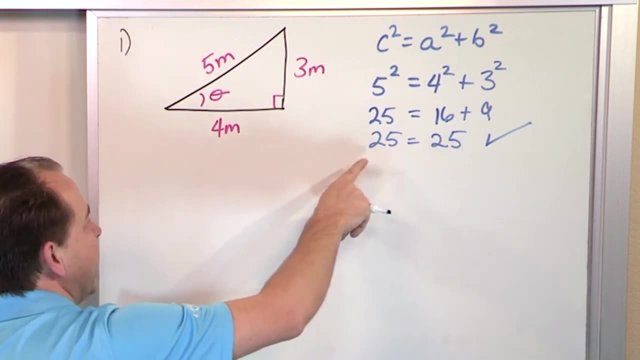 here. So this is 25, and this is 16, and this is nine. So 25 equals 25.. Check: If you ever get an inequality, like if you have 25 and this were a 22,, then something's. 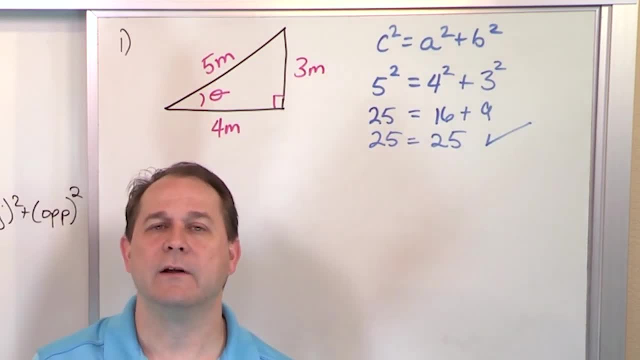 wrong, because the triangle has to be a right triangle in order to even use these sine cosine and tangent definitions. And if this thing doesn't work out, then this is not a right triangle, because the Pythagorean theorem always is true for a right triangle. 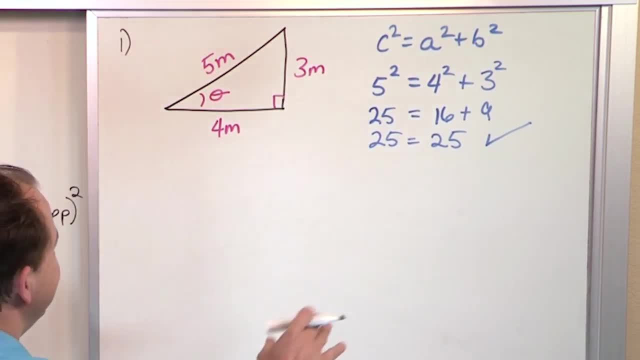 Okay, So this was just an aside. I wanted to show you the Pythagorean theorem works, but what I mostly want to do is I want to ask you the question: what is the sine of theta? So, literally, when this happens, you go back to your definitions, which we just wrote down. 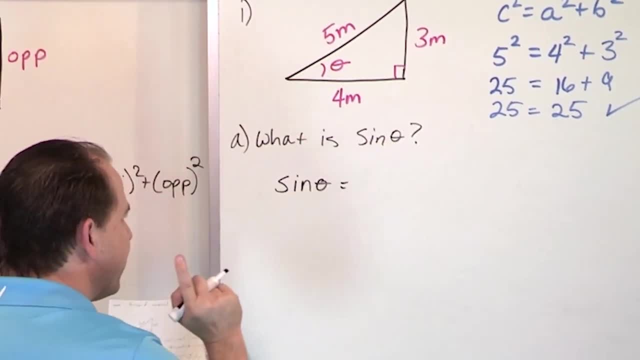 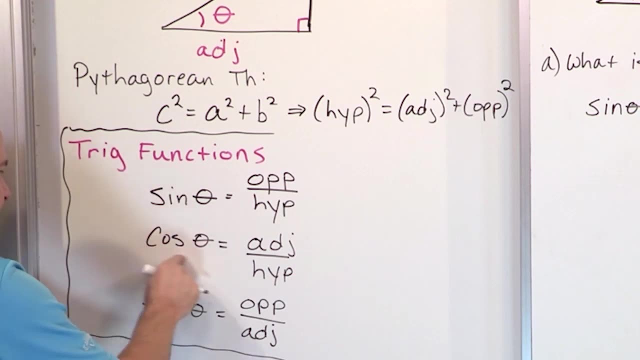 so I'm going to write it down again: The sine of theta is equal to you, remember? I want you to remember, if there's one thing in this lesson, remember that the sine of an angle involves the opposite side. Okay, The cosine of an angle involves the adjacent side. 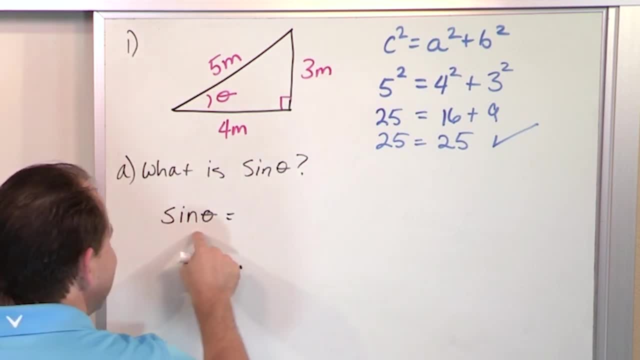 You're going to find out why that's so important as we solve problems. The sine involves the opposite side of this triangle and of course, it's divided by the hypotenuse: Okay, Opposite side, opposite to what It's opposite of this angle. 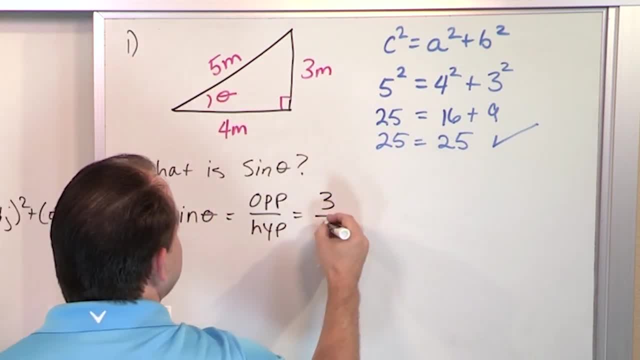 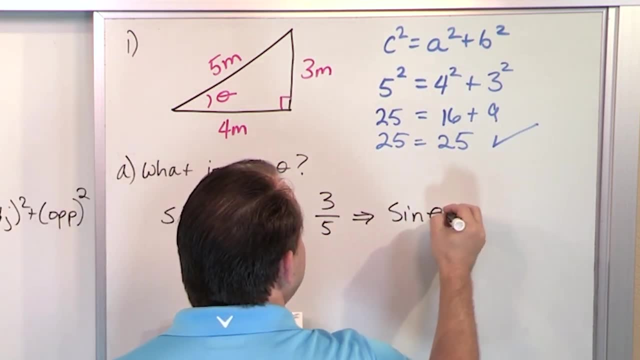 So that means it's three. The hypotenuse is the longest side, which is five. All right, So what this means is that the sine of this angle is equal to three-fifths of an exact fraction. If you put that in your calculator, you'll find that it's 0.6.. 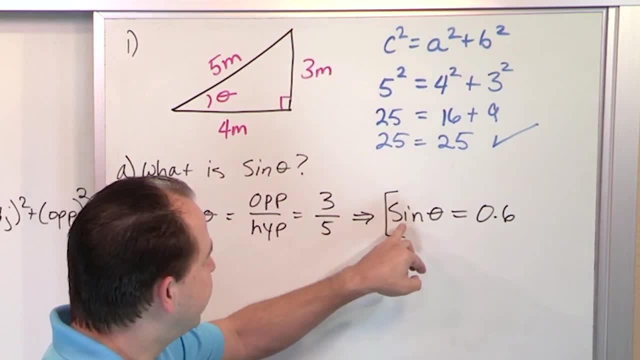 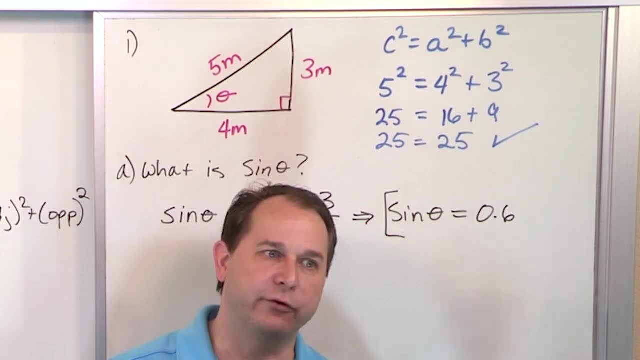 So if I asked you what is the sine of theta, you would circle this: The sine of theta is equal to 0.6.. All right, Let's go work the next part of this little simple problem, and then I'll circle back. 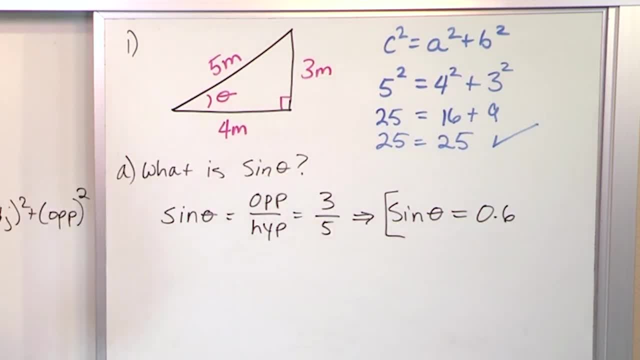 and draw some conclusions at the end. So that was for sine of the angle. Let's calculate for part b. let's calculate the cosine, You know what? Let's do it like this. Let's do it like this. Okay, Let's do it like this. 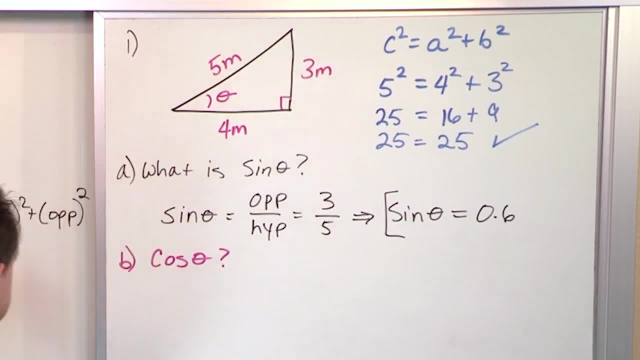 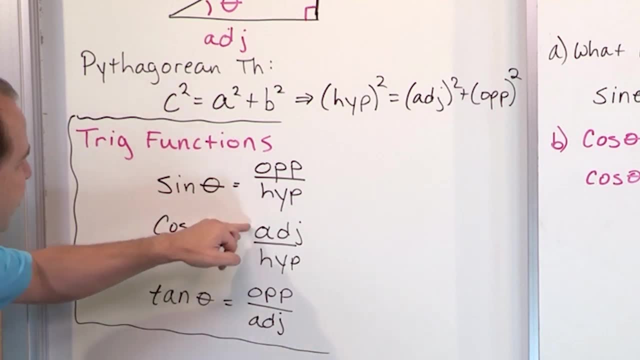 I want you to find the cosine of the angle. That's the question there. So what is the cosine of the angle? And I told you before, the cosine involves the adjacent side. So sine involves opposite, cosine involves adjacent. Try to burn that in your mind. 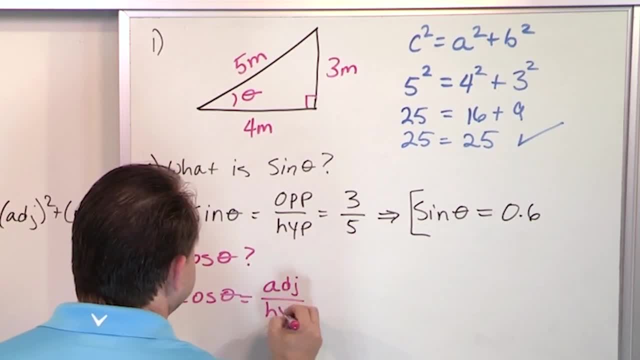 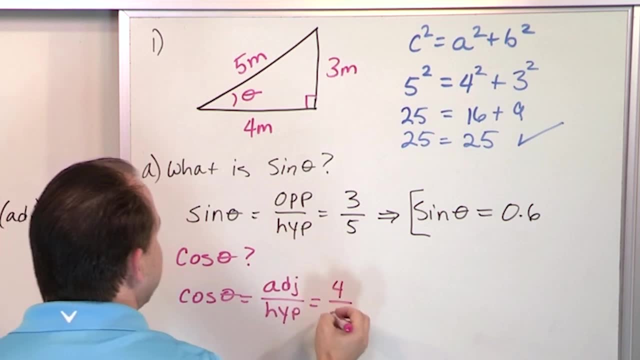 So you're going to write that down adjacent and it's going to be divided by the same thing, the hypotenuse. So you go back to your triangle. The adjacent side to this angle is four and you divide it by the same hypotenuse, five. 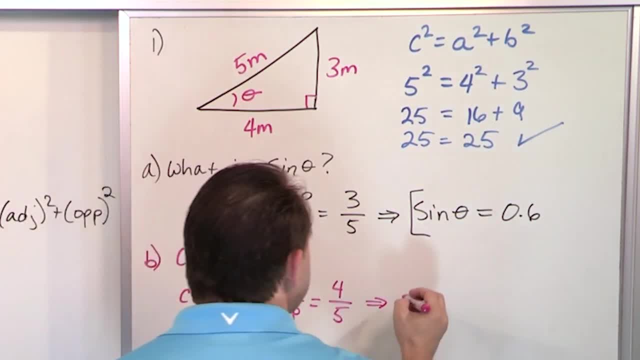 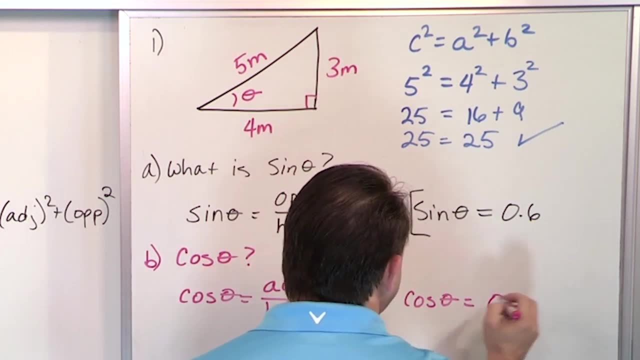 So it's an exact fraction four-fifths. So you would write down that the cosine of the angle theta is exactly four-fifths and if you want to put that in your calculator, you can 0.8.. That's the answer. 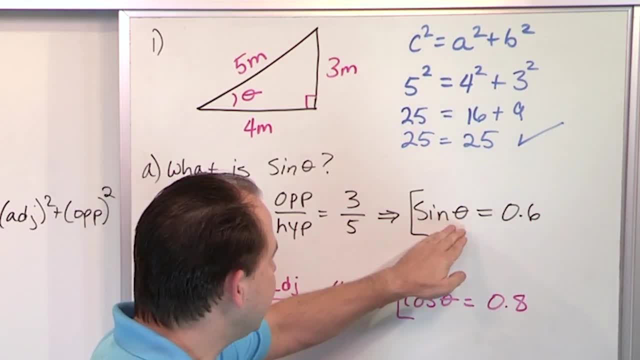 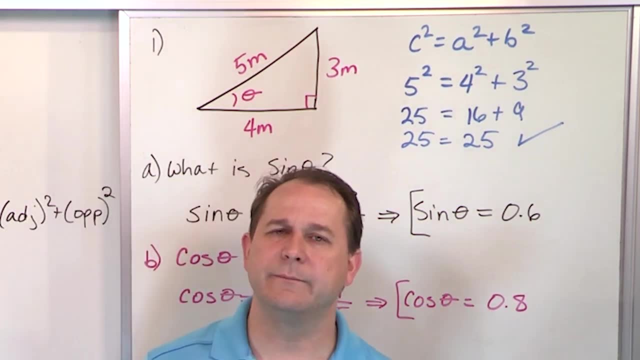 So notice first of all, before we go any farther. the sine of the angle came out to be some kind of decimal less than one, And the cosine of the angle also turned out to be some decimal less than one. That's always going to be true. 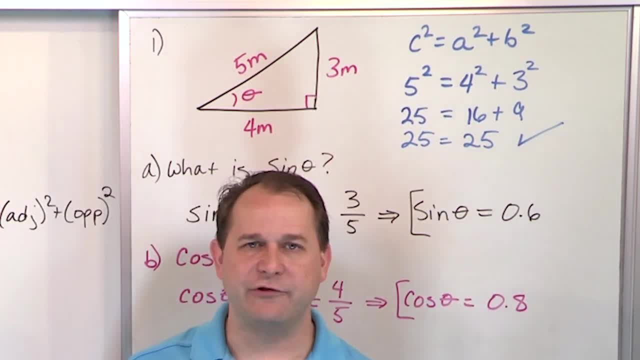 Right. So the sine Go. take your calculator out right now. Make sure it's in degrees or degree mode, because there are different modes in the calculator. We're going to be using degrees in physics almost all the time. If you take any degree angle you want, stick it in your calculator and hit the sine button. 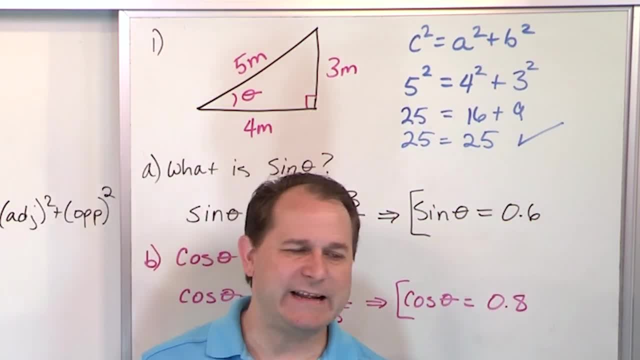 you're always going to get a number less than one. If you stick any degree number you want, any number you want, and put it in the calculator and hit the cosine button, you're always going to get a number less than one. That's going to be important to understand. when I wrap this all up in a nice bow at the 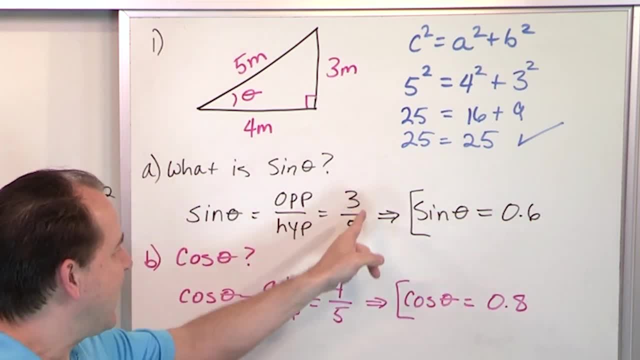 end. But you should always get decimals for these guys, Why? Because they're fractions And because we know that the hypotenuse is always the longest side of this triangle and the hypotenuse is always going to be on the bottom then whatever on the top is always. 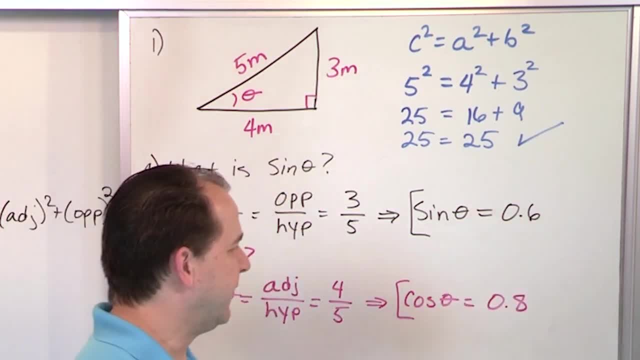 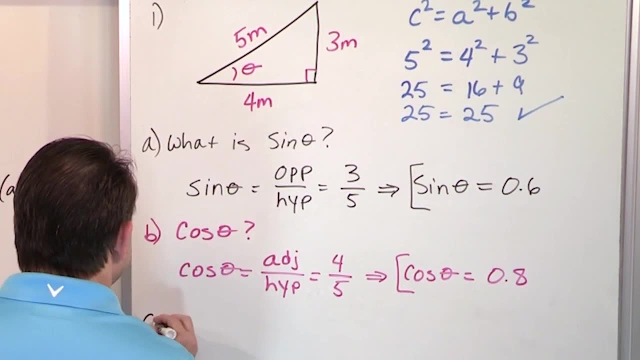 going to be smaller than the bottom, And that means that the fraction will always be less than one. So sine and cosine never get bigger than one, ever. That's the bottom line. All right, what is? Let's look at part C. What is tangent of this angle? 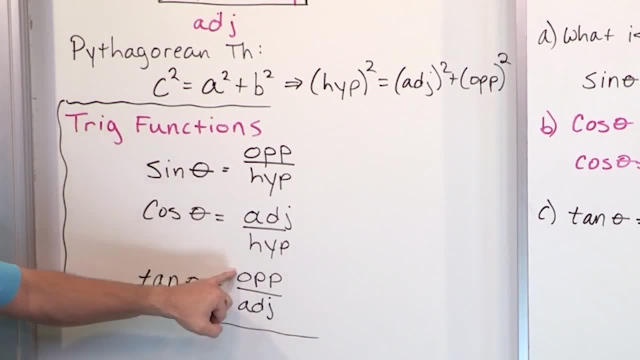 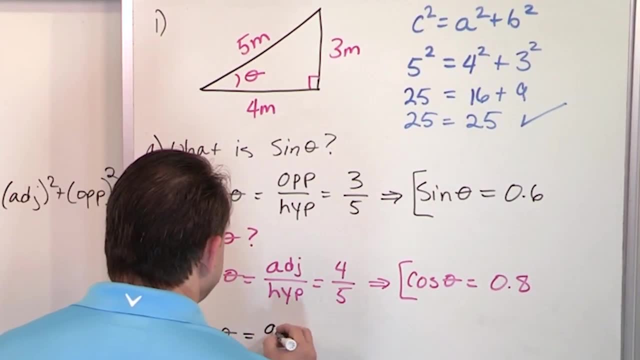 Tangent is defined as a mixture of the two. Tangent is the one that involves the opposite side, but it also involves the adjacent side. but there's no hypotenuse anywhere here, So we just write down the exact thing that we know. 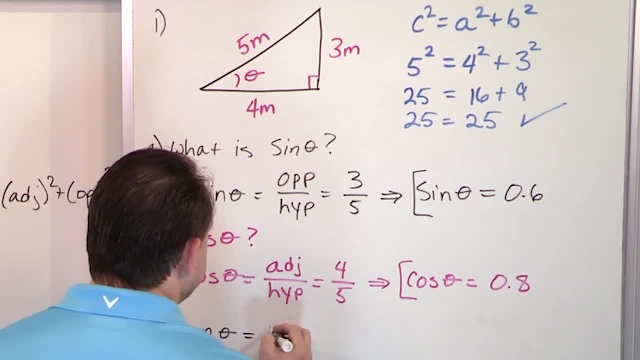 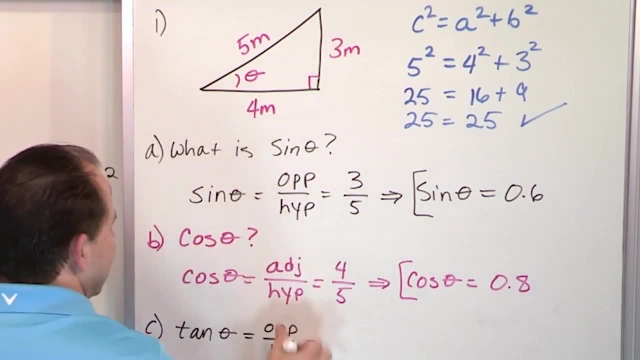 It's the opposite Whoops, I almost wrote down adjacent. It's the opposite side- over the hypotenuse. Opposite side is three Whoops, not over hypotenuse. Opposite over adjacent. Sorry about that. Opposite over adjacent. 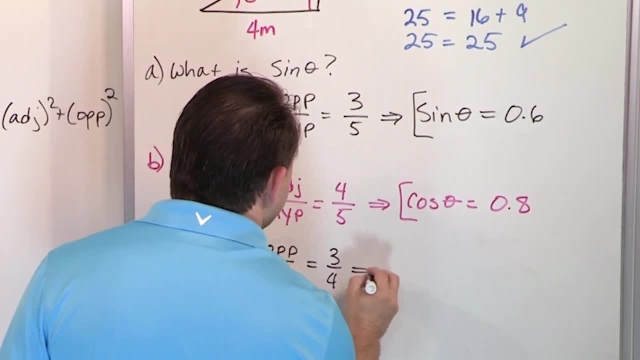 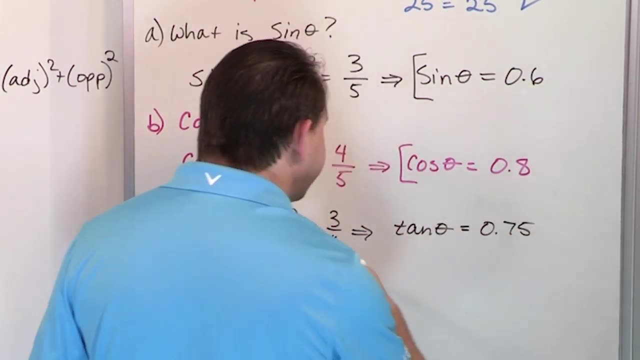 Opposite is three, adjacent is four, So three fourths. And you all know that that's 0.75, so you would write down that the tangent of some angle theta is 0.75, or you could write it as three fourths. that's fine too. 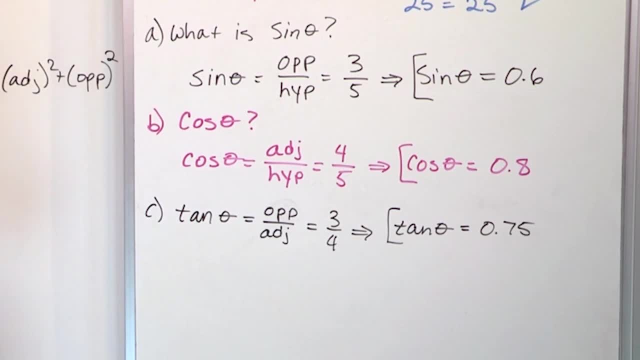 When there are exact decimals like this. I'm okay with decimals, so you can go put it there, All right. so now we know what the sine of the angle is, what the cosine of the angle is, what the tangent of the angle is. 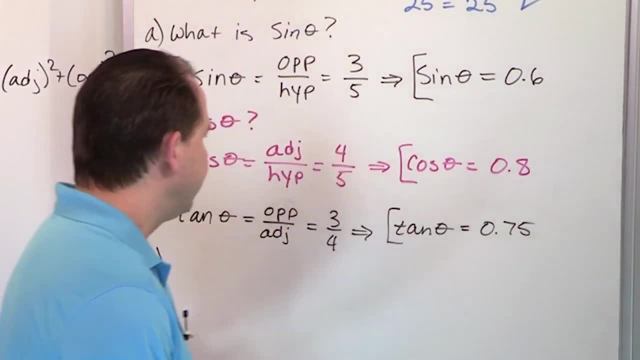 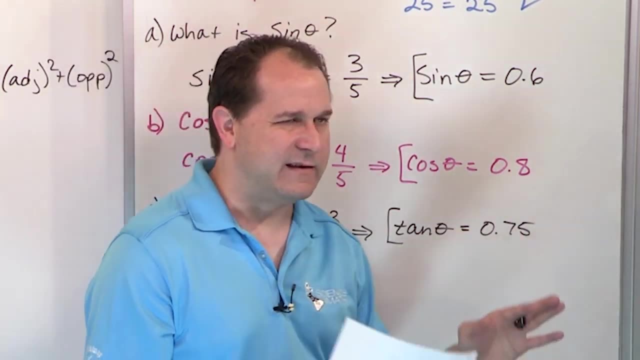 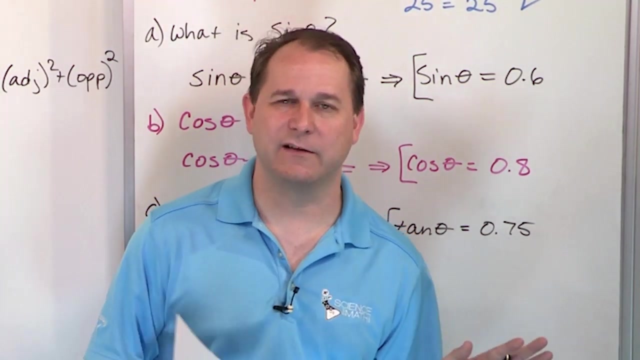 Also notice. the tangent of the angle is also less than one. For this example, the tangent's less than one. Now it turns out that the tangent function is not always in between, Is not always like less than one or whatever. The tangent function can go off the rails when you plot it. 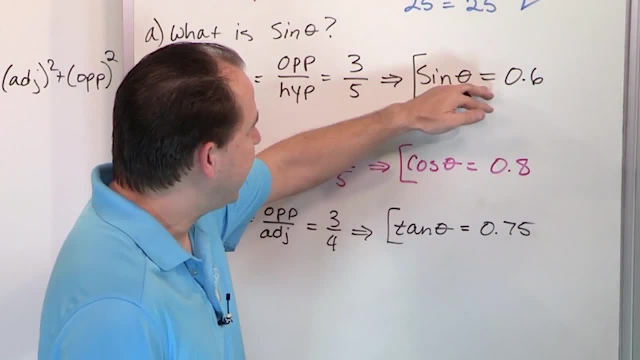 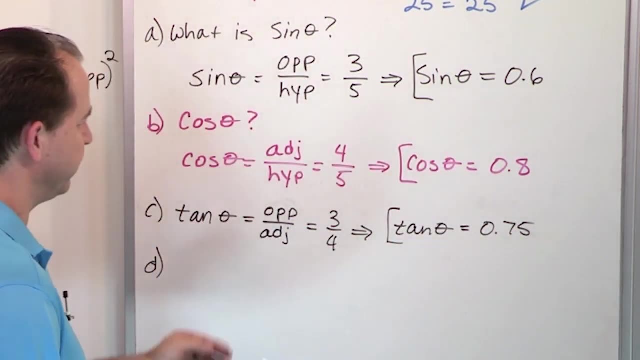 I'll explain that some other time. But for sine and cosine they always stay between plus one and minus one. okay, I didn't graph it for you, but it's plus one and minus one. This guy can kind of go all over the place and I don't want to get into the reason why. 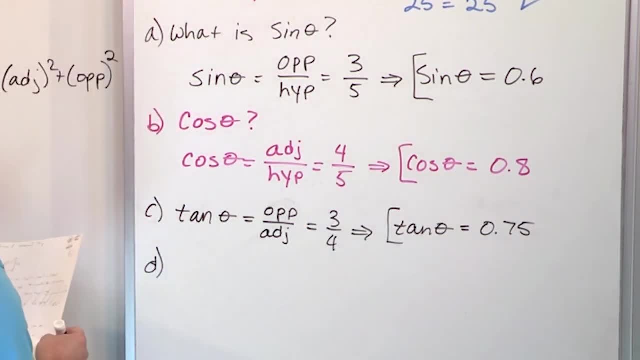 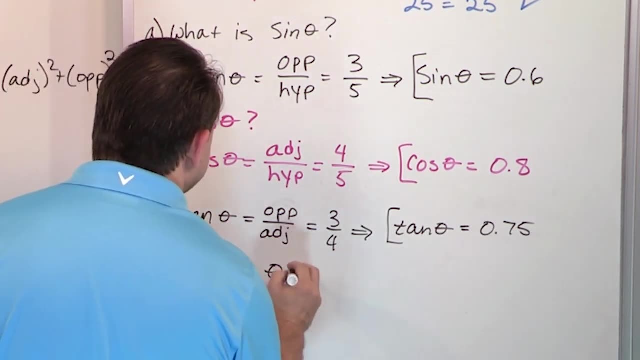 right now, but that's just something you can observe when you plot it. So let's find out the most important thing here: What is the angle theta? In other words, is this angle 13 degrees? Is this angle 17 degrees? 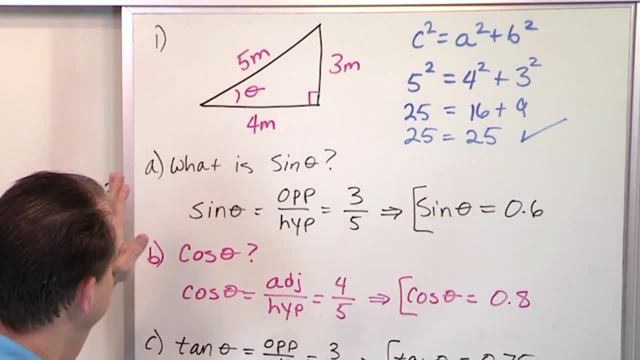 Is this angle? 35 degrees? What angle is it? The first thing I want you to know before we actually calculate the angle is: this angle is locked in place by the distances of this triangle. In other words, if you got some string out or a pencil and you measured five and you 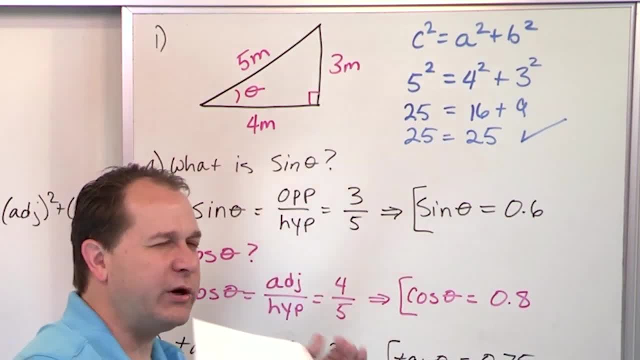 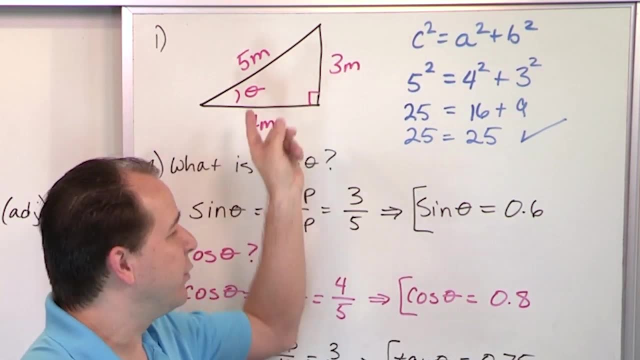 measured four and then you went up vertically and measured three. there would only be one way that you could put those together to make an actual triangle that connected. That one triangle would have an angle here. That would be fixed. It's fixed because the sides of the triangle are locked in place and you're arranging. 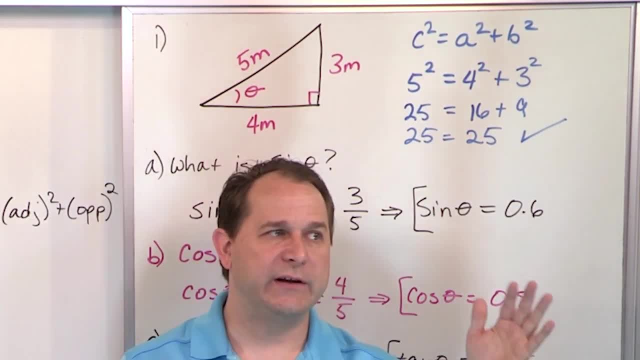 them in one way, because they have to make a right triangle. So for any given set of sides, there's only one angle. There's only one answer. I just don't know: Is it 35 degrees or is it 42 degrees? 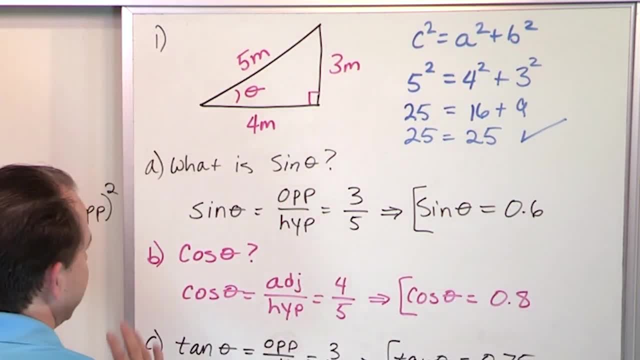 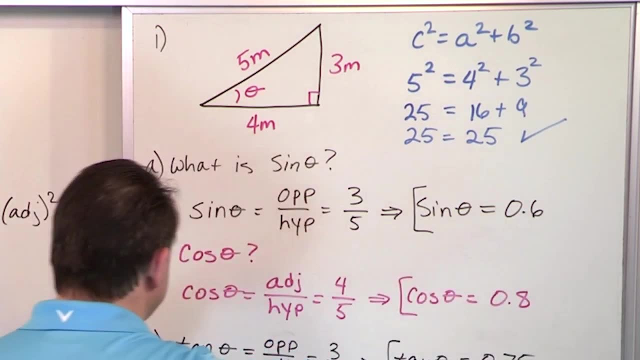 What is it? And so the way I figure it out is. there's lots of different ways, but the first one is: Let's go back up here. We calculated what the sine of the angle here was, and it was 0.6.. 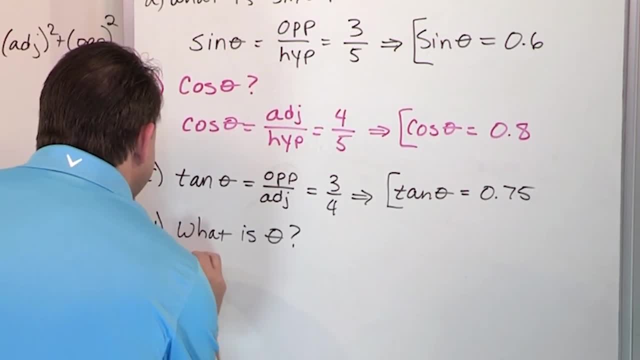 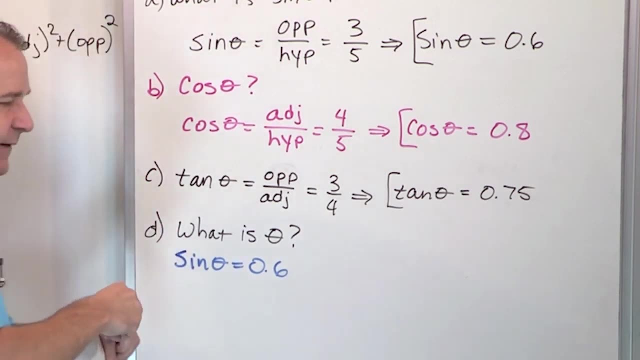 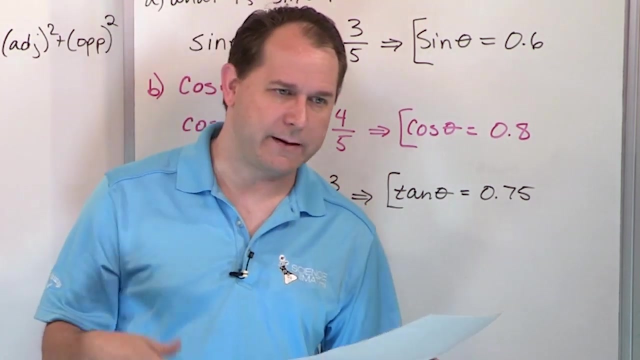 All right. So we know that the sine of this angle is 0.6.. We calculated that before. So remember, from equations, from equations like algebra equations, you do the opposite. to solve for x, right, You might divide by something, multiply by something, add by something, get x by itself. 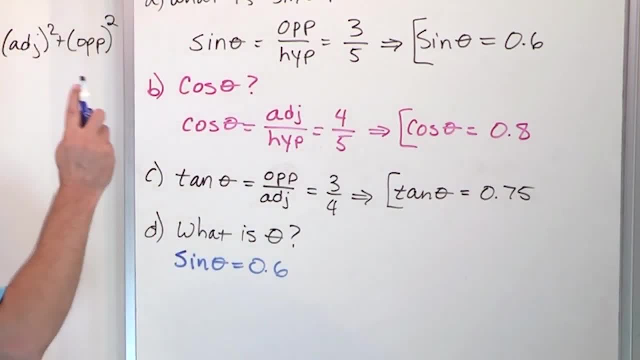 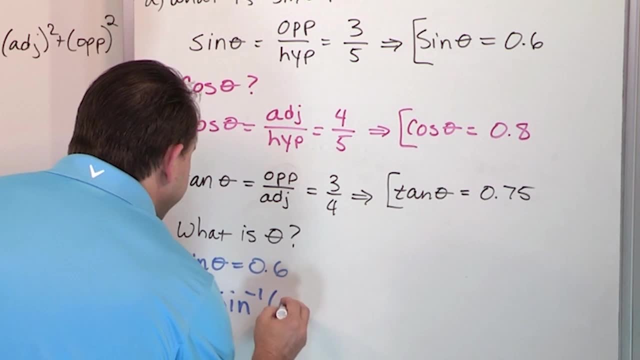 But the angle that we want to find is wrapped up in a sine. How do we do that? Well, we say: well, the theta is going to be equal to. We have to do the inverse function, In other words, we have to undo it with an opposite. 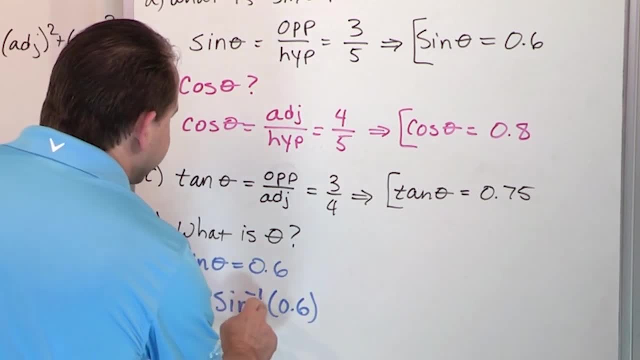 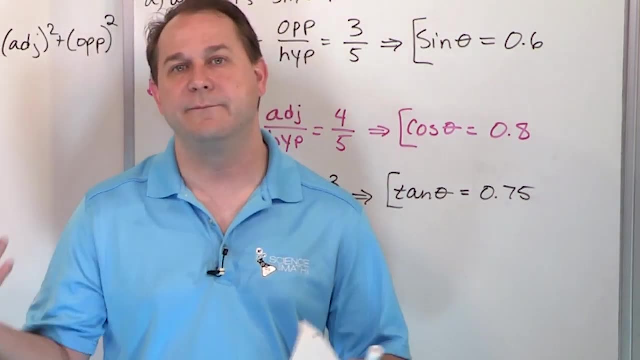 So if sine is the function, inverse sine. that's what the negative one means. This is inverse sine or arc sine. you might see it undoes it. So like the opposite of addition is subtraction, The opposite of multiplication is division, when solving equations, 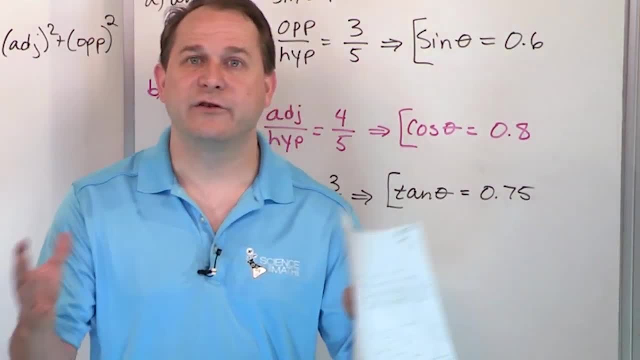 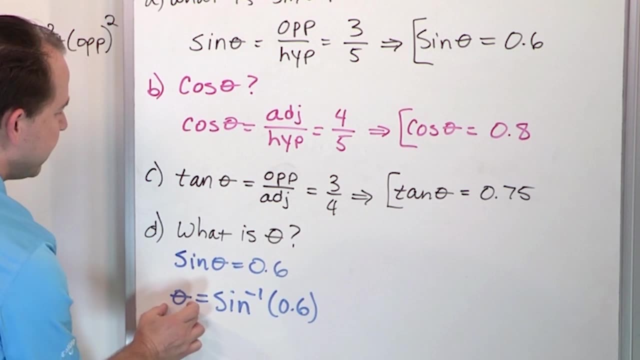 The opposite of squaring something is a square root. The opposite of sine is inverse sine right. So when we do inverse sine to both sides of this thing, inverse sine on the left undoes it. so we have theta. Inverse sine on the right is what we're writing here. 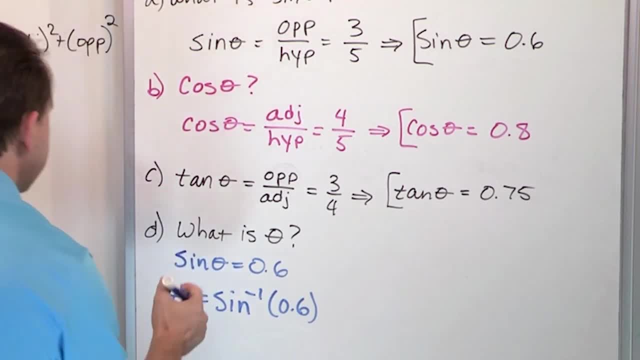 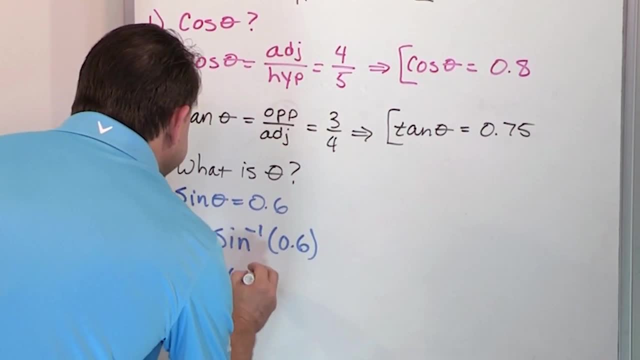 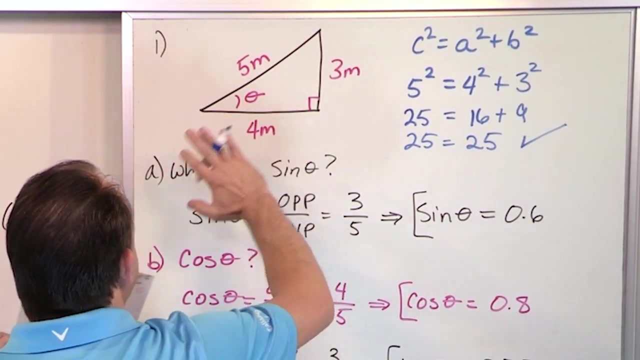 So if you stick 0.6 in your calculator and hit the inverse sine button, you're going to get the angle back and the angle in this case is going to be 36.87 degrees. So that's the angle. So if you built this triangle, this would be 36.87 degrees and it can't be any other. 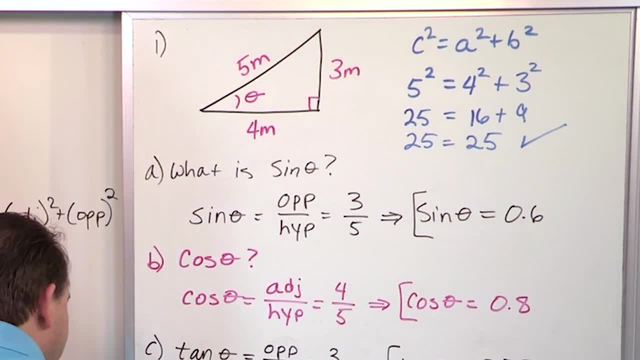 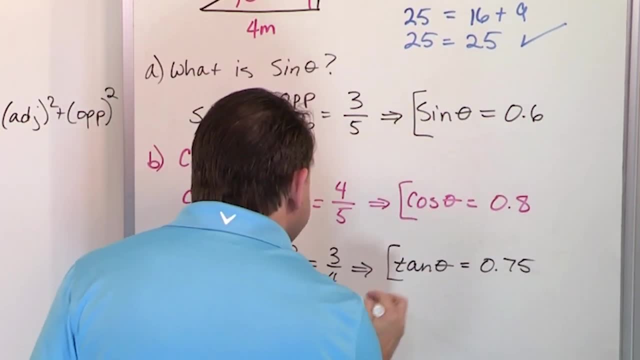 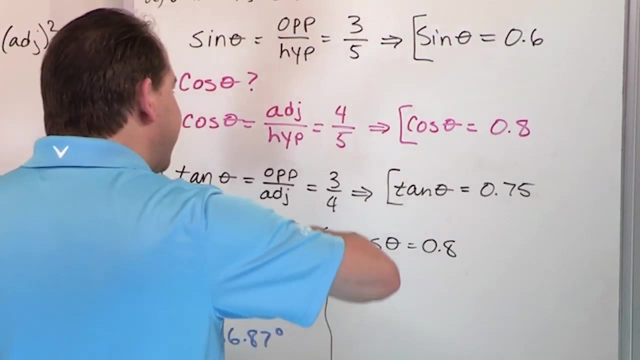 angle, or else you can't make the triangle. to begin with Now we calculated theta using the sine, but we can actually calculate it using the cosine, because we also learned for this triangle that the cosine of the angle is 0.8.. So if we want to get theta by itself, we have to inverse cosine both sides. 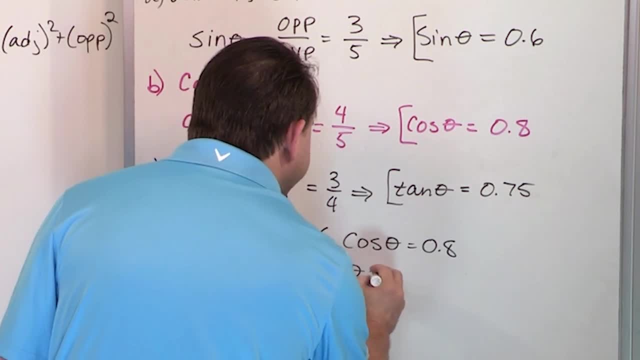 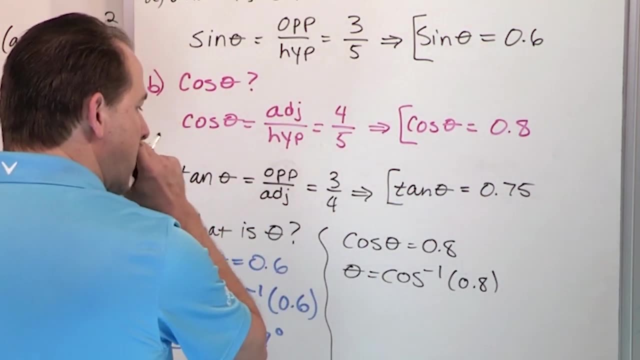 That eliminates. it kind of annihilates the left-hand side, leaving theta by itself. It'll be the inverse cosine 0.8.. So if you put 0.8 in your calculator and find the inverse cosine button and hit that one, 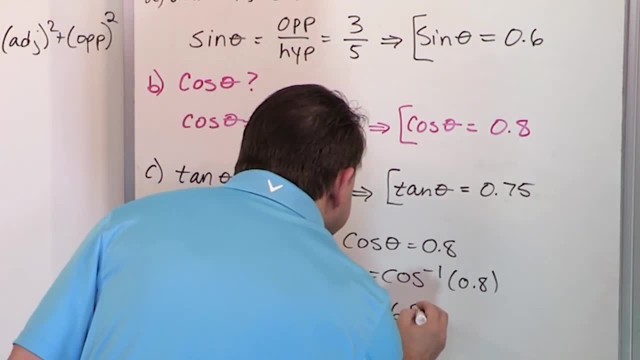 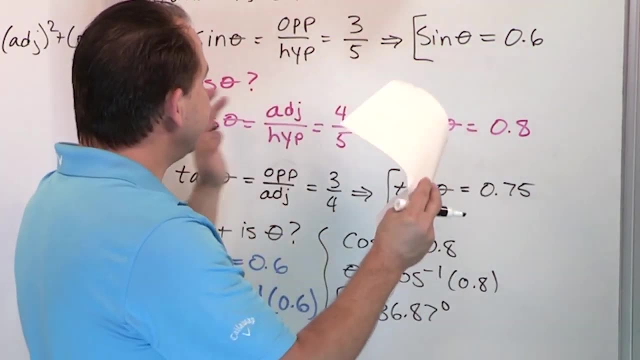 what do you think you're going to get? You're going to get 36.87 degrees. 36.87 degrees- Notice it matches exactly, Okay, Exactly. Everything's self-consistent, whether you use the sine to find the angle or the cosine. 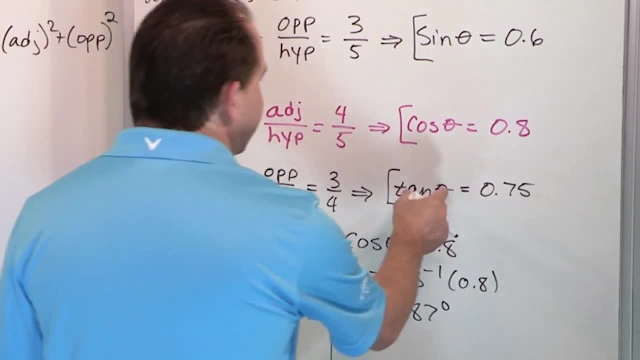 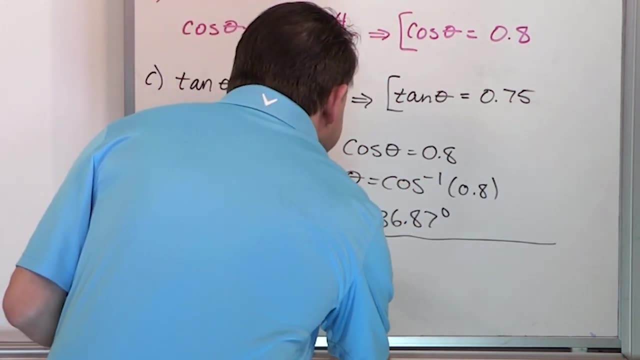 to find the angle, you get the same thing. Now, what do you think is going to happen if we use the tangent? So let's go here just kind of squeeze it in the bottom. If tangent of the angle is 0.75, then the angle should also be. what do you think? 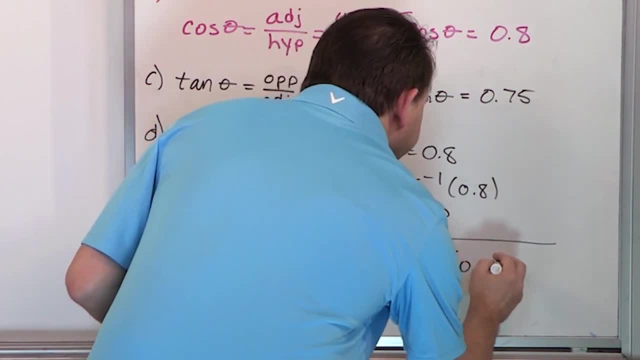 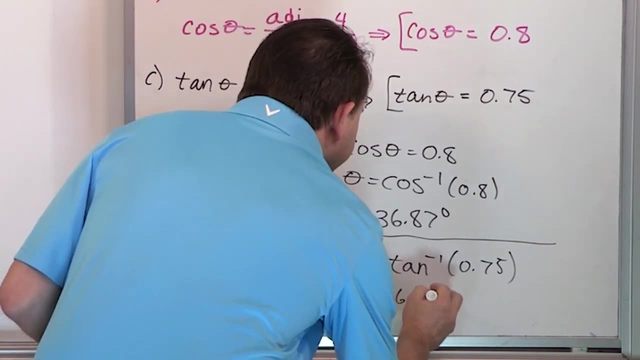 The inverse tangent of 0.75.. So if you put 0.75 and find the inverse tangent button, what do you think you're going to get? You're going to get 36.87.. The purpose of this example was two things. 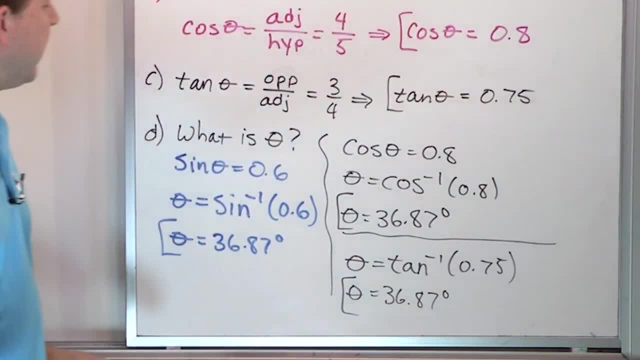 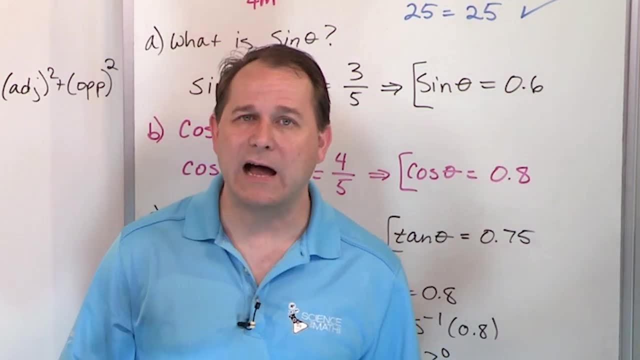 To show you how to calculate sine cosine tangent and to show you that you can take any one of these things and do its inverse: to find the angle. all right, Because you're going to be finding the angle a lot, A lot of times it'll be. here's what a baseball's doing. 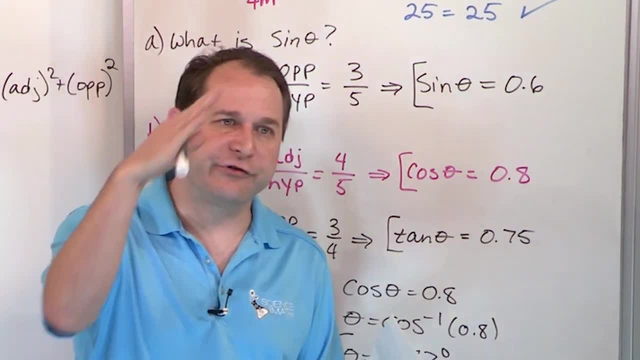 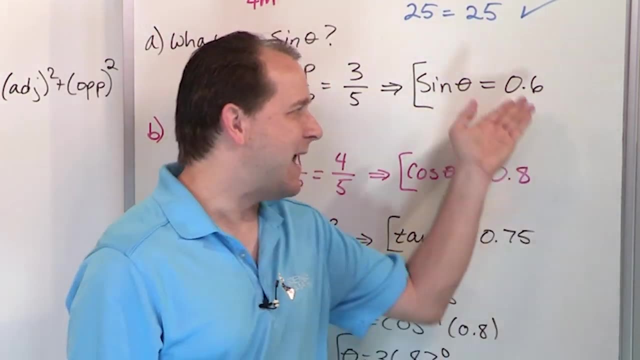 What is the angle? What angle did you throw it at? Well, eventually you're going to construct a triangle and you're going to end up having to figure out what this angle is, and you'll use one of these. So the second part of this is to tell you that it doesn't matter which one you use. 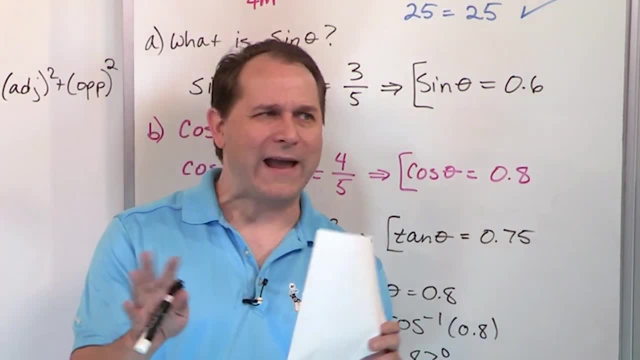 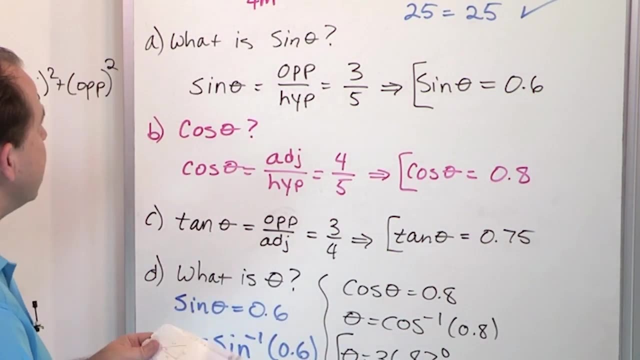 They all give you the exact same answer. So there's not so much a right way to find the angle, It's just there's about 16 different ways- not literally, but there's a bunch of different ways to find the angle, okay. 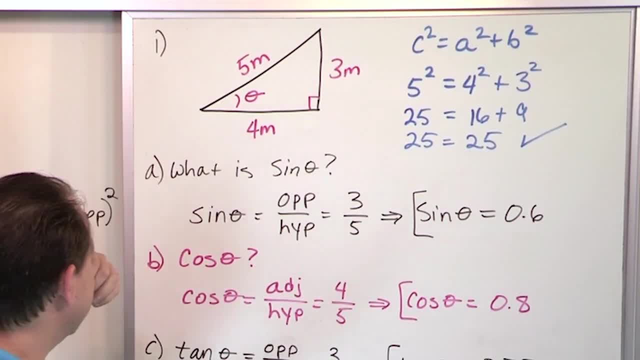 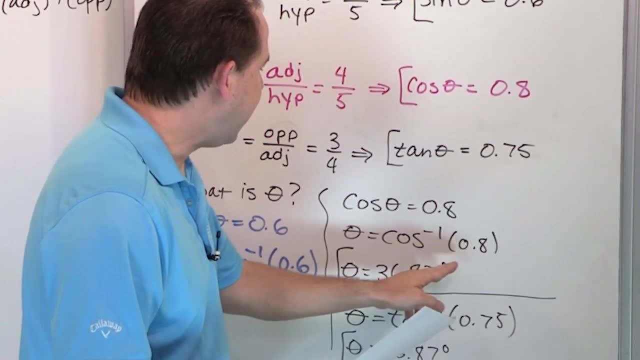 The only other caution I want to throw at you when you're dealing with triangle trig like this is this: angle is when you put these numbers in a calculator like 0.8 and find the inverse cosine, you do this inverse tangent and so on. when you do this stuff, the angle 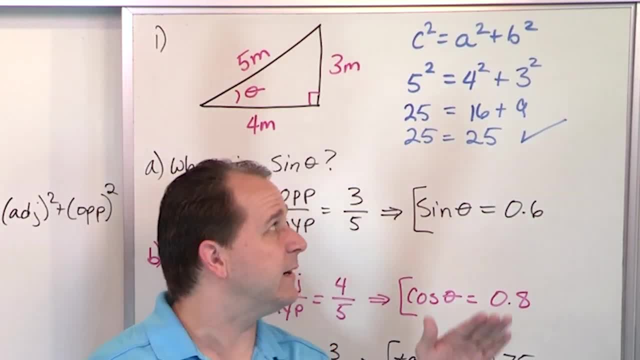 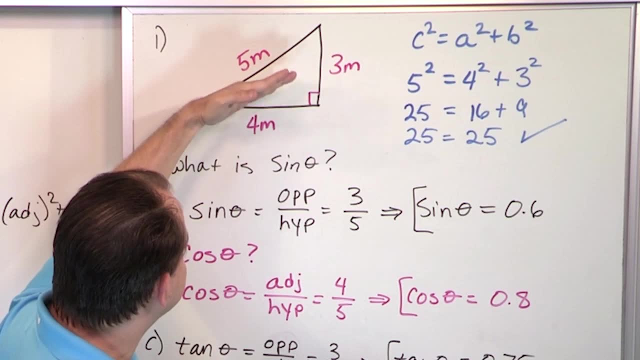 that your calculator's going to give you is always going to be the positive angle. It's always going to be the angle as if the triangle was drawn here, and it's going to give you this positive angle. This is a positive angle because it's measured from the x-axis, like this: 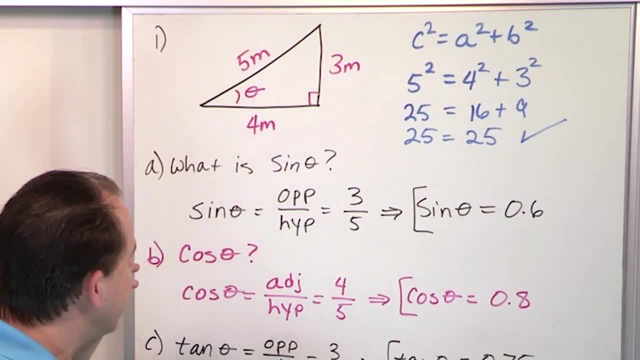 This is x-axis, y-axis, so this is a positive angle. right As we go and do more problems, I'm going to caution you: when you're inverse tangenting or inverse cosine or inverse sine, you've got to be a little careful because you have 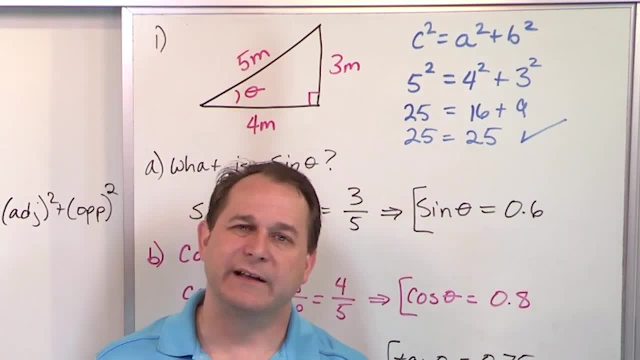 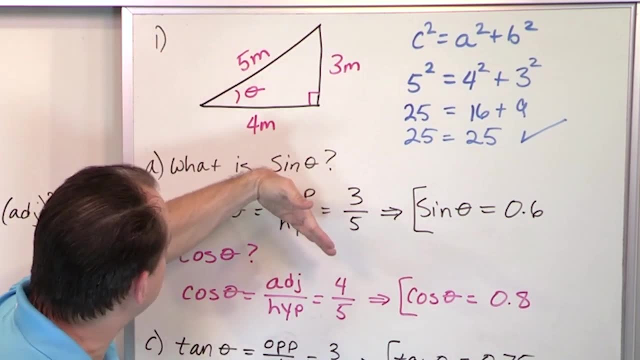 to know that that calculator's always going to give you the positive angle. Because sometimes, what if I'm throwing the ball down right? So the triangle's not oriented up like this, it's oriented down, and that means that I'll actually have a negative angle. 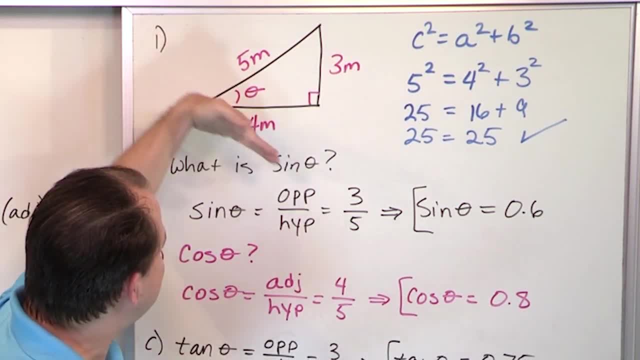 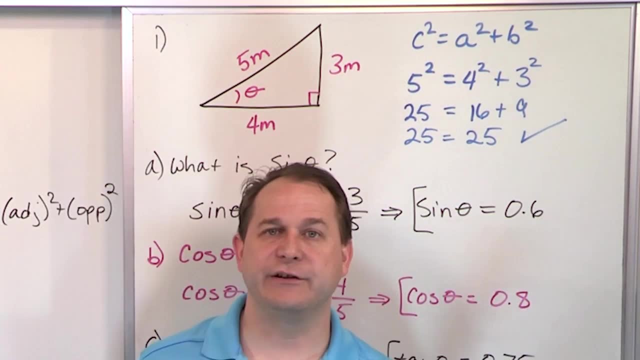 Okay, There's a negative value for the y and a positive value for the x, And so, long story short, you've got to be careful to look at the quadrants of what you're actually doing When it returns that angle. you just have to know that it's always going to give you. 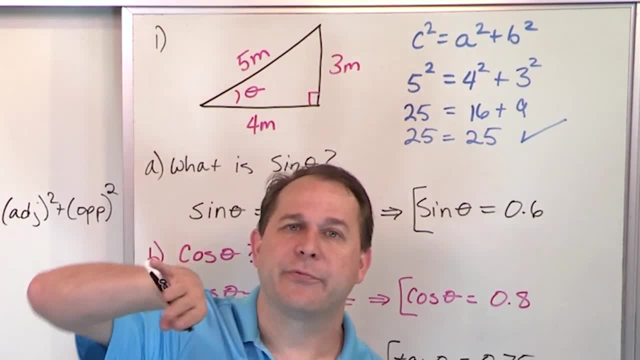 that positive angle, But your problem might actually be throwing the ball the other way and you might actually have to add 180 degrees to that angle or something like that to get the correct angle you want. But when we get to that point, I will explain and caution you as we do. more problems like 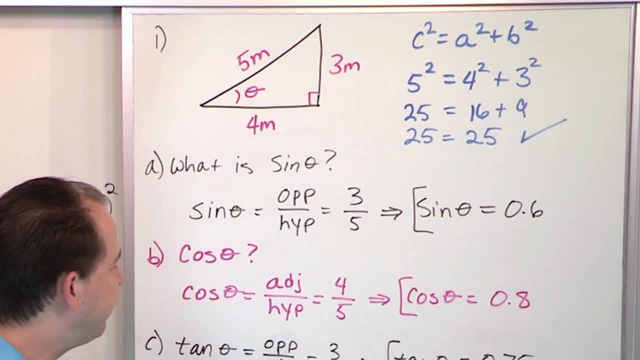 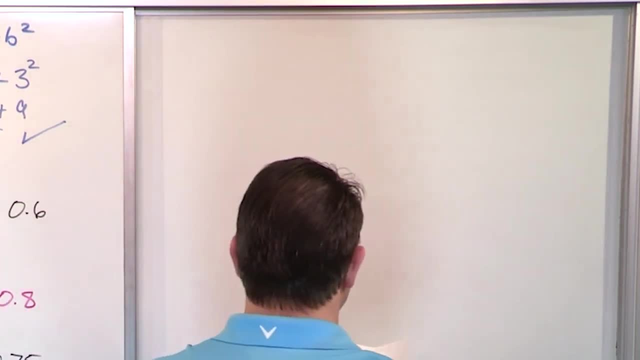 that For now. just know, When you inverse cosine, inverse tangent, you're always going to get that positive angle back. That's all I want you to remember at this point. All right, so this is very important. coming up next: 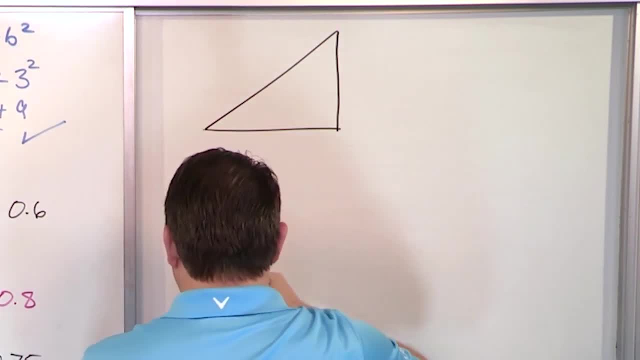 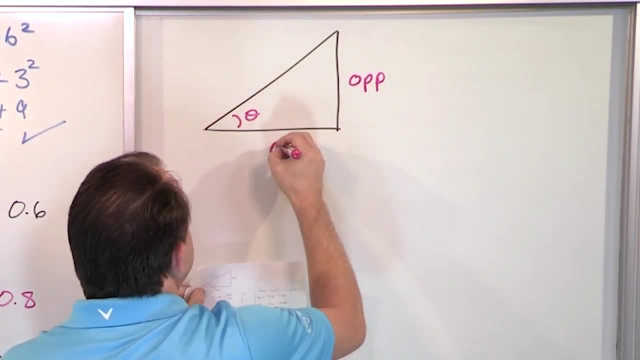 If you have a triangle, as we have been talking about, and it has some angle, theta, and it has an opposite side, and it has an adjacent side and it has a hypotenuse, as they all do, I'm kind of regurgitating over. 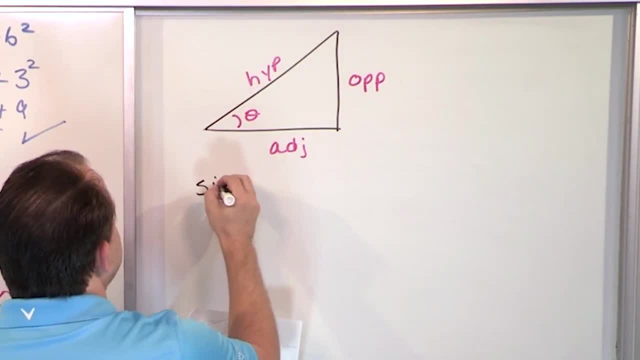 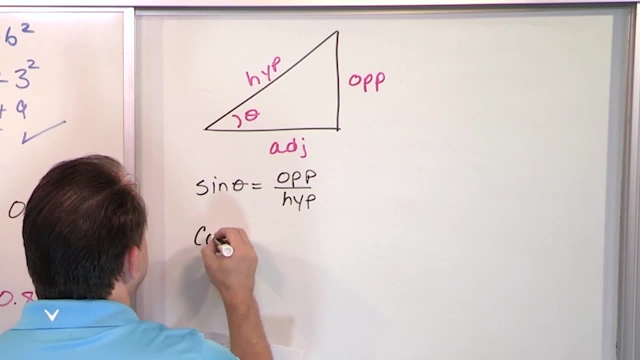 And over again that we had talked about the fact that the sine of the angle was equal to the opposite- Remember, sine deals with opposite over hypotenuse- And we talked about the fact that the cosine of the angle had to do with the adjacent side. 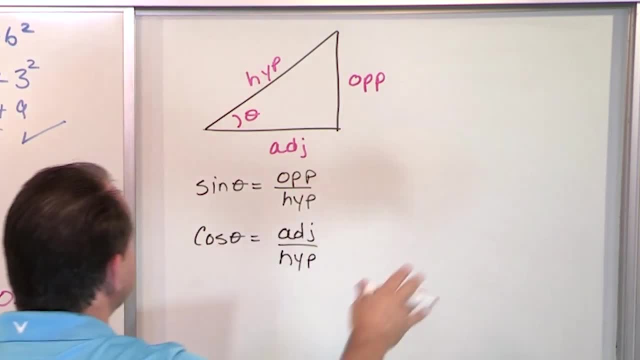 Remember cosine deals with adjacent over hypotenuse. Absolutely true, But there's actually a little bit. I don't want to call it easier, but it's a very, very useful way to write this down If you were to take this and solve it for the opposite side. 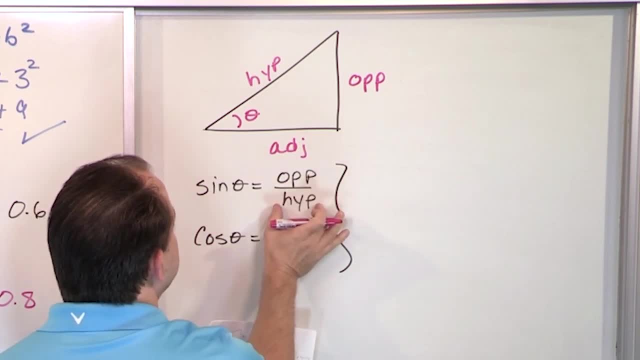 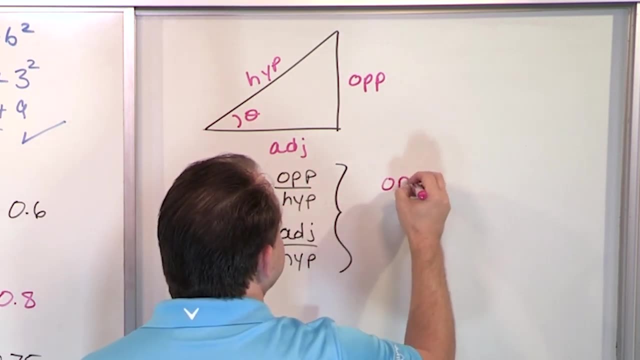 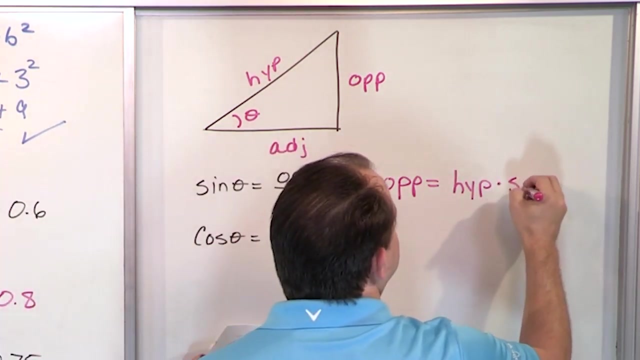 How would you do that? Well, this is a fraction. You have to multiply left and right by the hypotenuse right. So if you solve this equation, you're going to see that the opposite side is equal to the hypotenuse times sine theta. 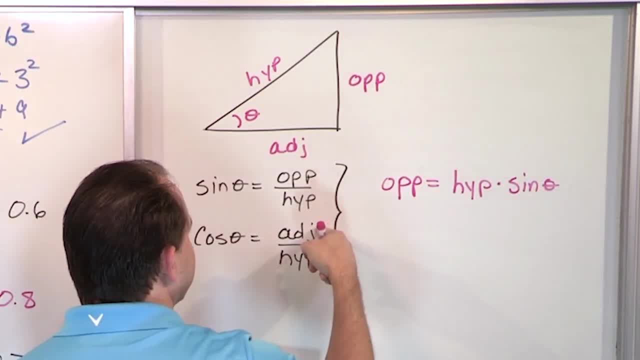 Let me do this one, and then I'll explain what I'm talking about here. also with this one, The adjacent side is equal to the hypotenuse times sine theta. Okay, Let me do this one, and then I'll explain what I'm talking about here. also with this one: 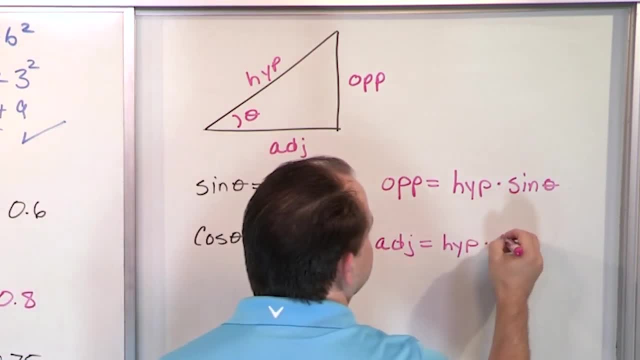 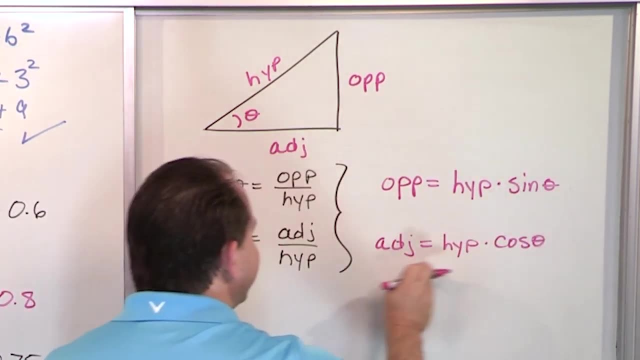 The adjacent side is equal to the hypotenuse times sine theta. These equations are the same thing as these. There's no difference. I'm not introducing anything new. I'm just telling you that if you take this relation and you solve it, for the opposite 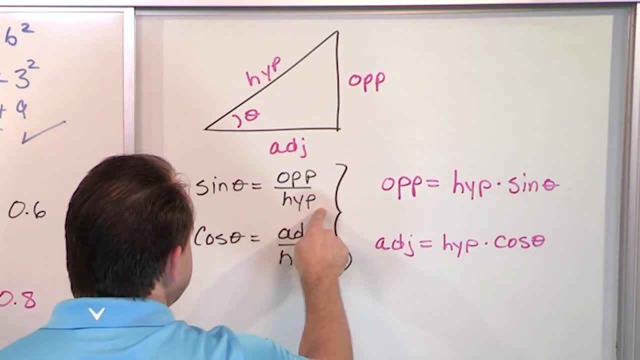 side, you'll have to multiply both sides by the hypotenuse, so it cancels on the right, giving you the opposite side. Here you multiply by the hypotenuse. Same thing here. Here you multiply by the hypotenuse. 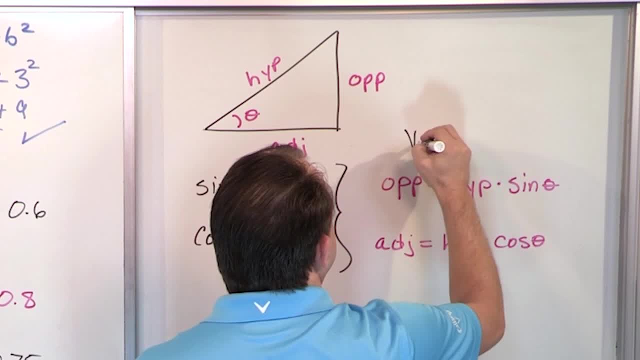 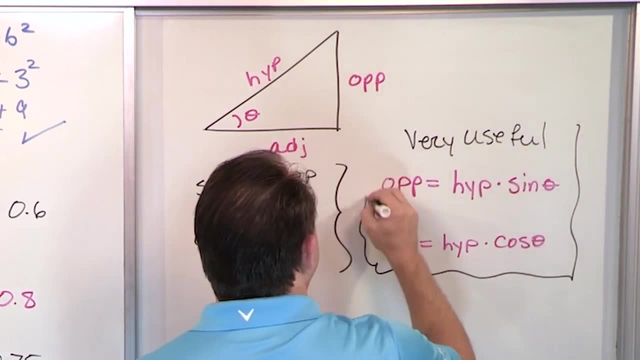 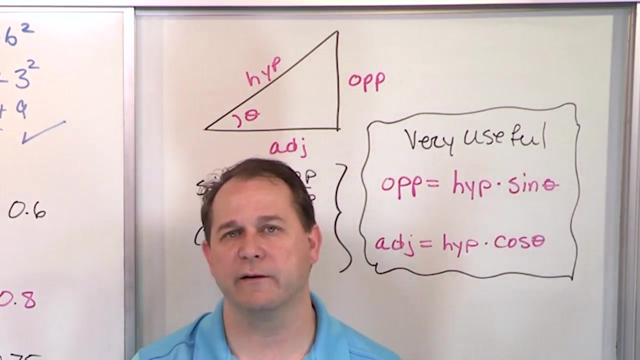 All right, These are very useful, All right, All right, Okay, They are the exact same thing as these. of course they are, but they are very useful. And the reason they're useful is because, in physics, we deal with something called a vector. 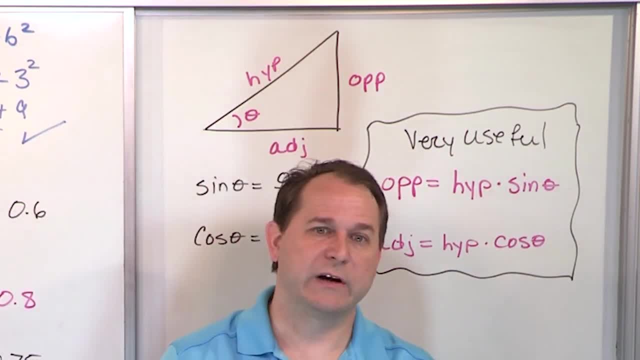 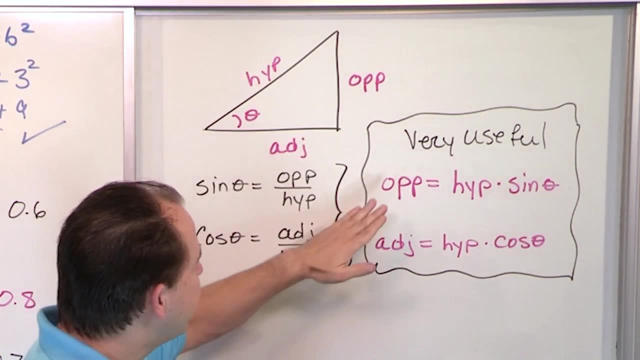 I'm actually going to explain really briefly what a vector is to you now, but then we're going to have an entire lesson, actually two or three lessons- on vectors. So don't stress out if you don't get everything right now. But the point is, these particular relations are very, very useful. 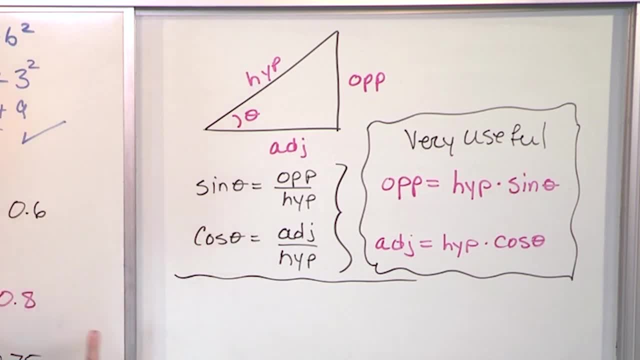 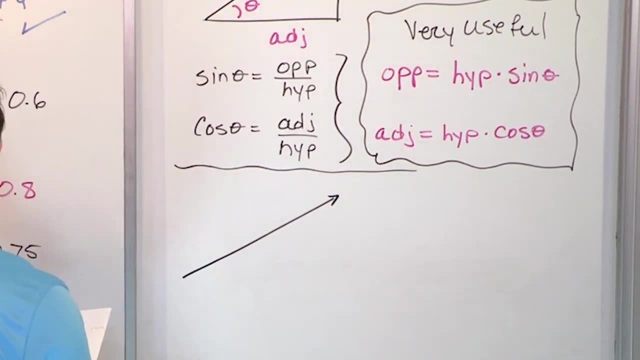 Let me explain why they're useful, because this is one of the very first things you'll be doing in physics. Let's say: I throw a ball this direction right, How fast do I throw it? 10 meters per second. Obviously, I'm not throwing it horizontally, I'm throwing it up with some angle. 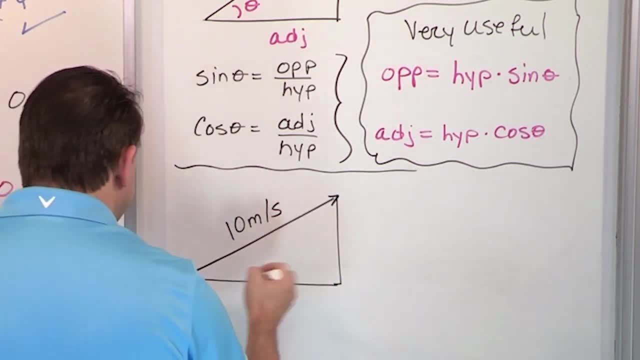 So what I do is I define the angle. and the way I define an angle is I draw a right triangle And I'm always throwing the ball relative to the ground. this is the ground here. So let's say, I throw that ball at 35 degrees. 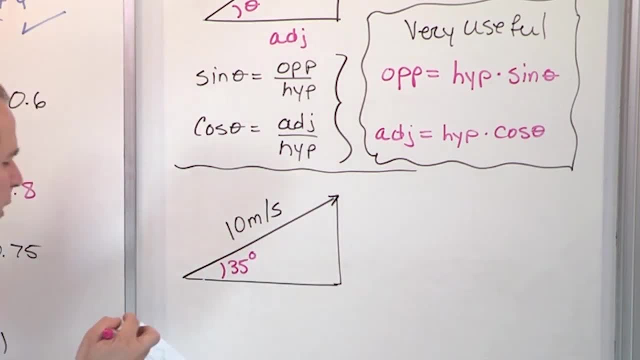 Let's put numbers in here instead of just theta. okay, You all know that if I throw a ball, If I throw a ball at an angle up, I have to throw it kind of in two directions, right, When I do that, I'm throwing it horizontally. that's the horizontal speed. 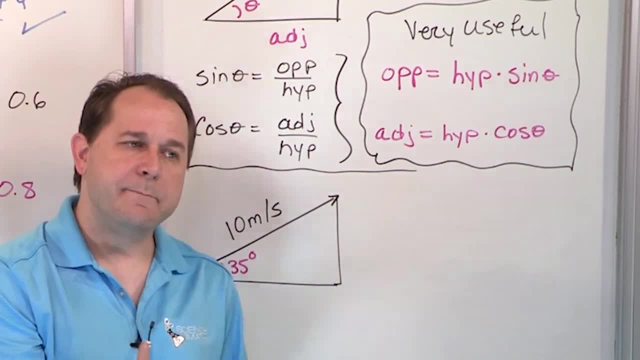 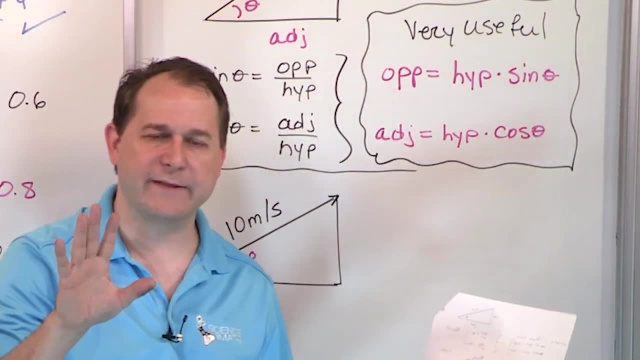 and I'm also throwing it vertically, straight up and down. The mixture of those two motions, horizontal and vertical, is what gives you the. I know the path curves, forget about the curving, but right when it leaves your hand, it's going at an angle which is a mixture of those two. 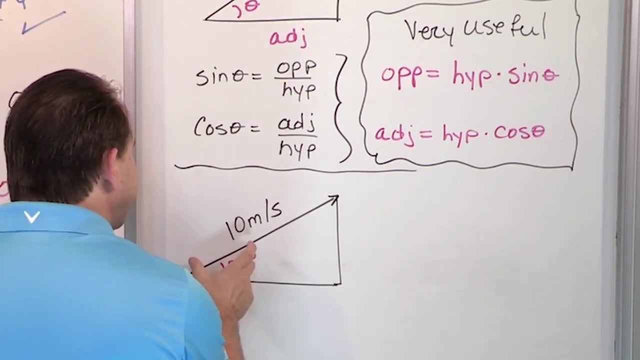 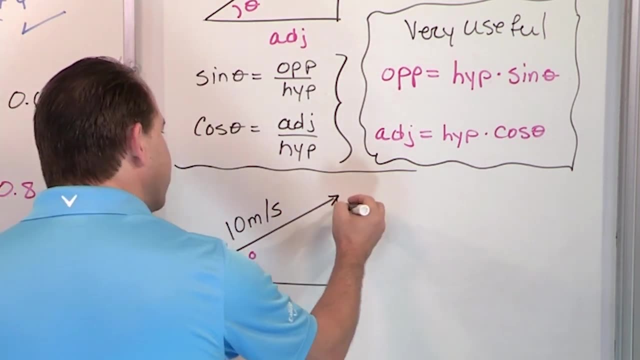 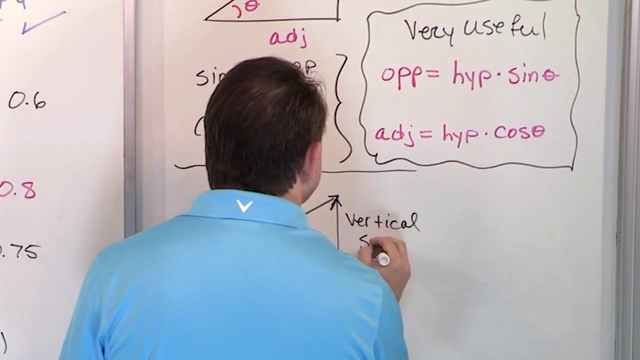 And that mixture is reflected in the triangle. You can see that if I throw it at 35 degrees, that the horizontal component of the velocity is bigger than the vertical component of the velocity, So I might have a vertical speed right. I know I've been throwing around the words speed and velocity. 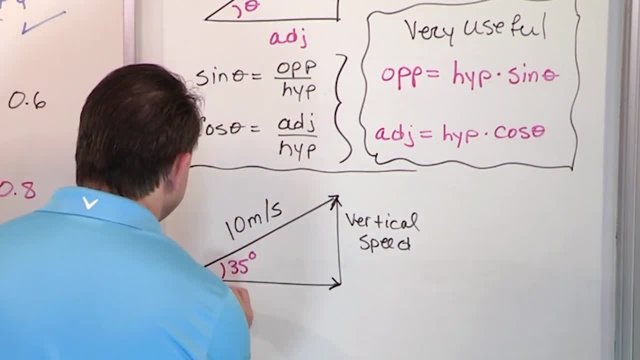 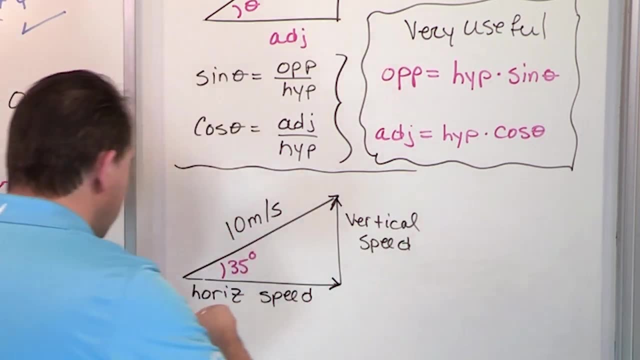 We'll define these terms a little bit, but I think all of you know that. what speed, more or less, is Horizontal speed? Okay, So the reason I'm showing you, The reason I'm showing you that these relationships are very useful, is because of the following thing: 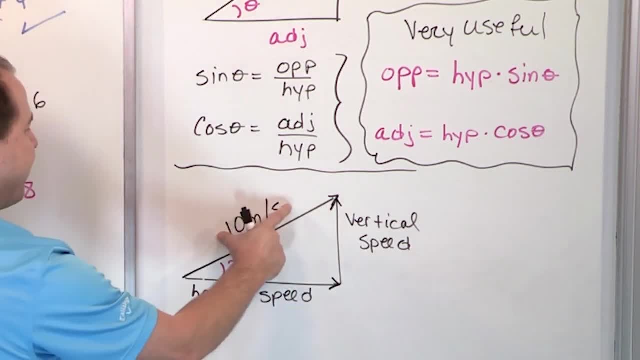 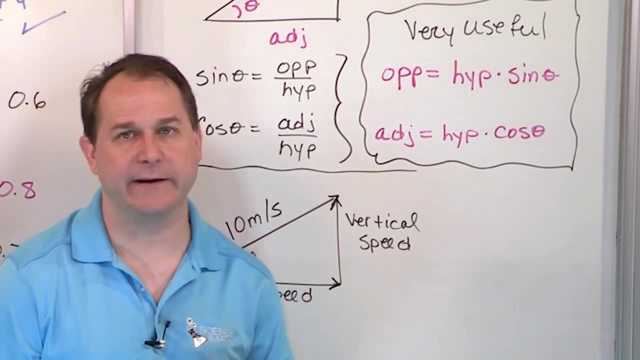 Usually I throw a baseball. this arrow represents how fast I'm throwing that ball. in total, in the angled direction, 10 meters per second. That's what that means. 10 meters every second that ball goes. That's pretty fast. That's faster than I can throw. 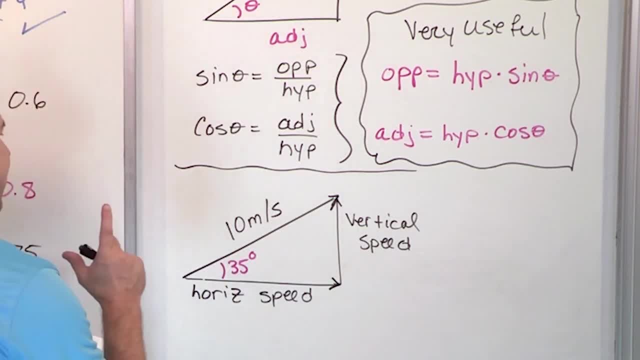 But anyway, it's a nice number. Okay, But let's say that I want to figure out what is the vertical part of the speed, In other words, how much of the speed exists only in the up and down direction and how much of the 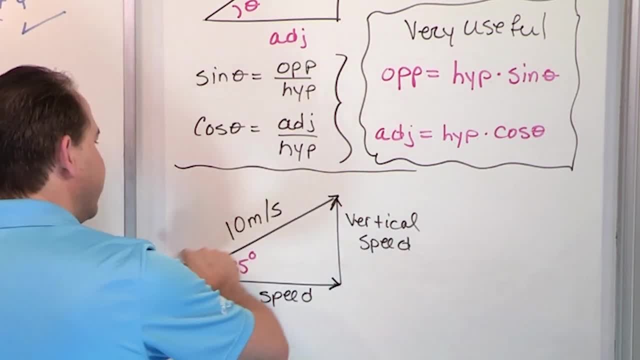 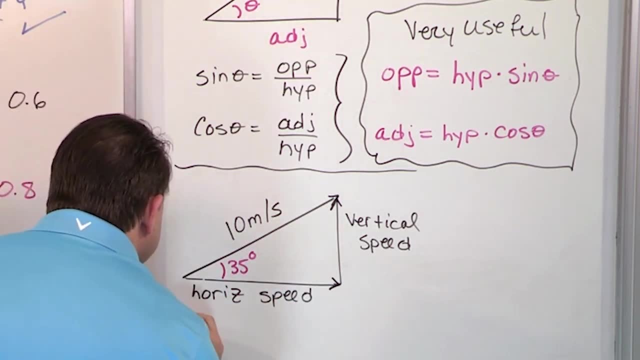 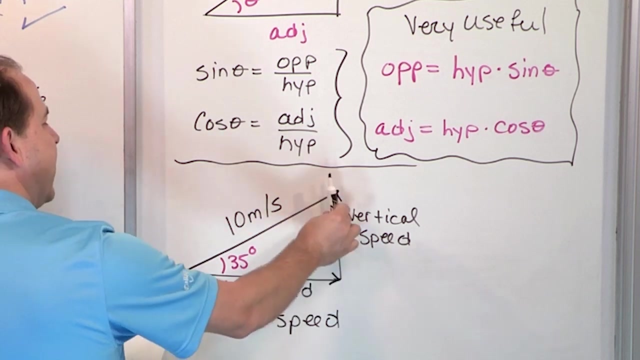 How much of the speed exists only in the horizontal direction, Because the angled speed is a mixture of the two. All right, So here's what you do: The vertical speed. Notice in this triangle: the vertical speed is the opposite side of this triangle to the angle. 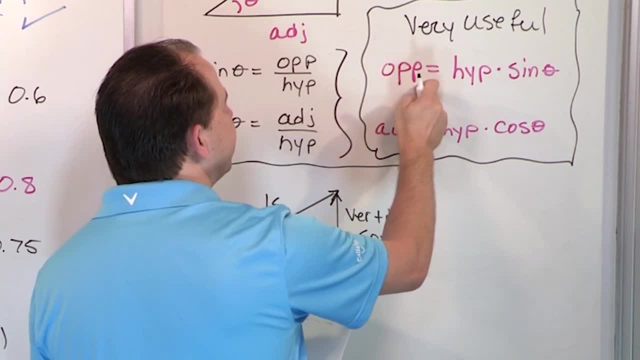 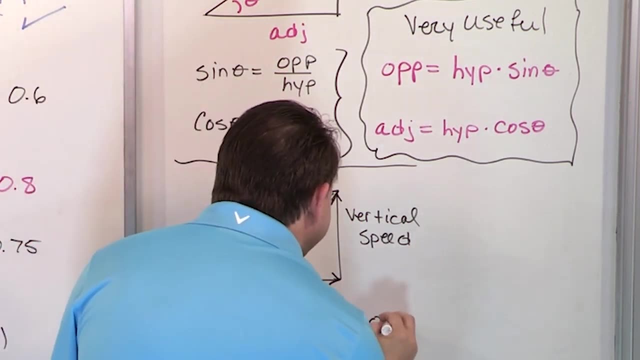 Notice that this equation tells me the opposite side of this angle, or the opposite side of the triangle, is the hypotenuse times the sine Right. So I'm trying to find The opposite side of this triangle, which I know from this equation: is the hypotenuse times the sine. 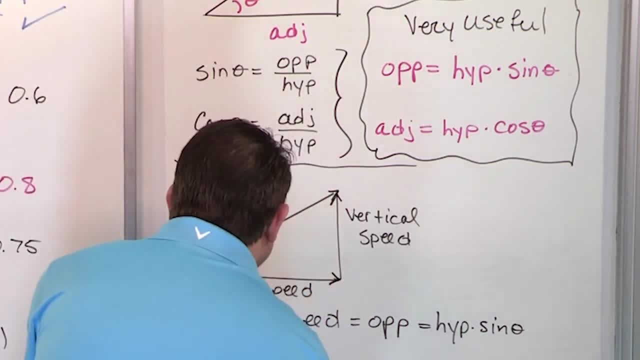 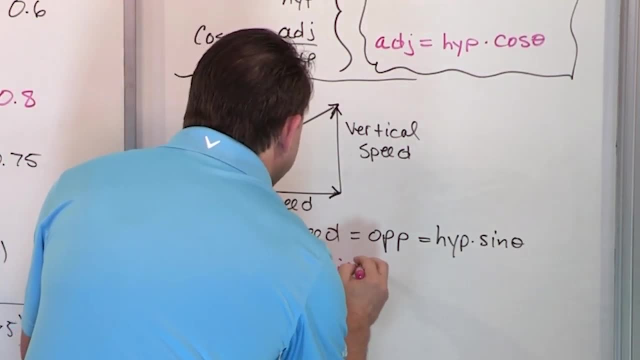 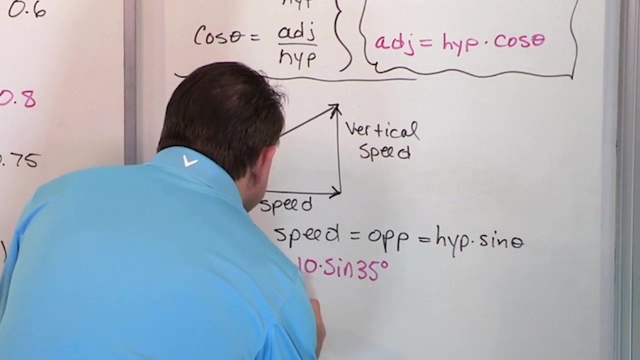 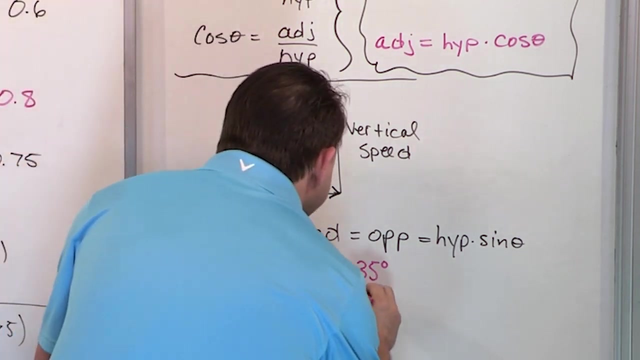 Okay, Which means that the opposite side of this triangle is equal to what? 10 times the sine of 35 degrees. Right? So the vertical speed is equal to: If you take sine 35 and you hit that in your calculator and you multiply that answer by 10, you get 5.74 meters per second. 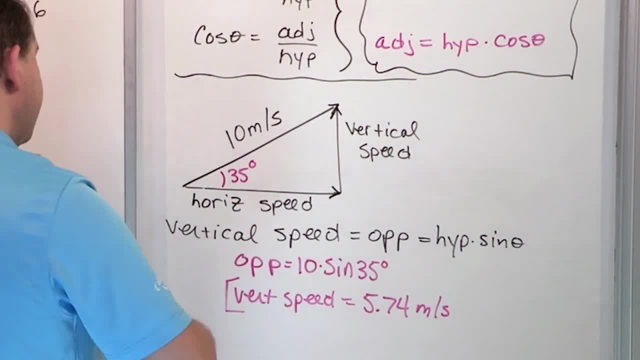 It's the same units as whatever I threw it with. Let me kind of leave that alone. Let's calculate the horizontal speed, and then I will wrap it all up together and impress upon you something that you really must remember. Okay, so the horizontal speed. 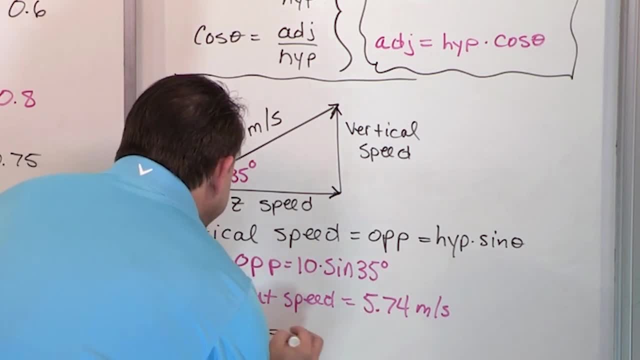 Horizontal speed. what is that? That's the According In this triangle. that's the adjacent side of this triangle. That's what I'm trying to find, The adjacent side of this triangle. But we just said, from this equation, from the definition of cosine. 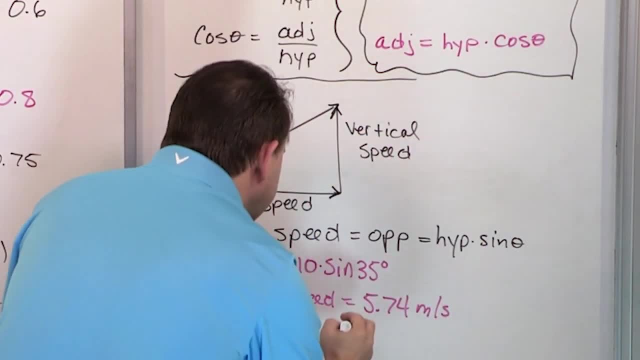 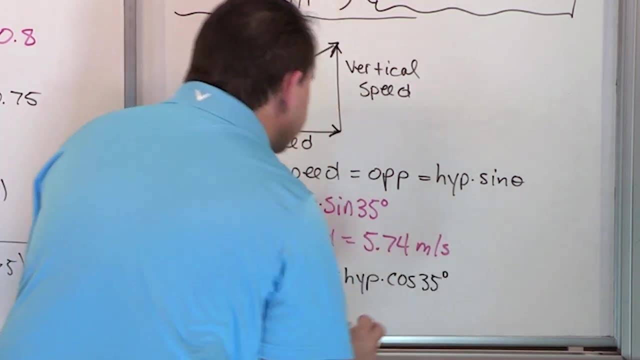 I can find the adjacent side of any triangle hypotenuse times cosine, So it's the hypotenuse times the cosine of. Now I know the angle is 35 degrees Right And so Let me switch colors to kind of put the point home. 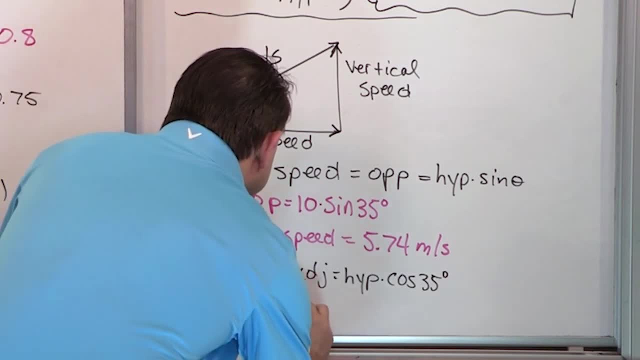 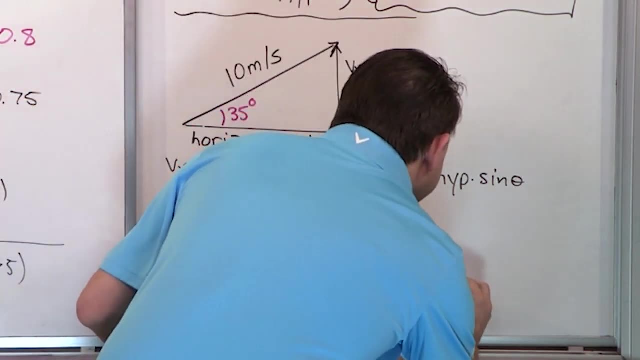 So the horizontal speed is equal to what It's. Well, the hypotenuse here is 10.. So let me, Let me go ahead and just write it down here. So it's 10 times the cosine of 35 degrees. 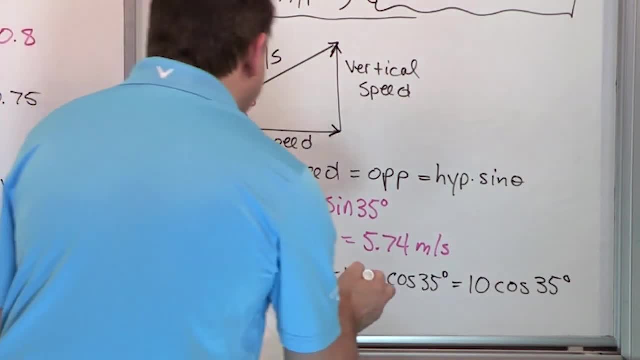 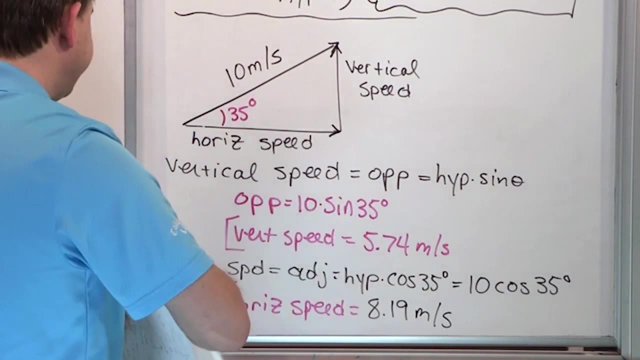 So if you take 35 degrees, hit the cosine button, multiply by 10, you'll get 8.19 meters per second. Now, first of all, let's see if this makes sense. We're saying that we're throwing a baseball at 10 meters per second at some angle. 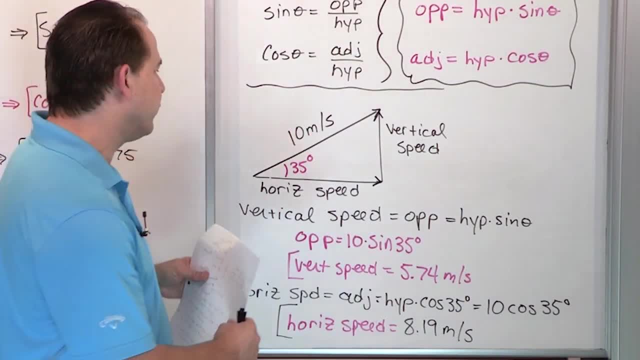 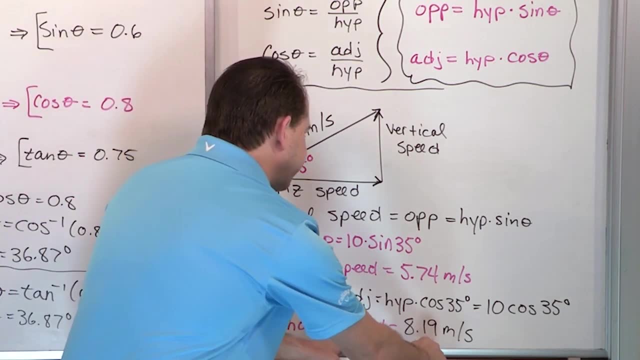 And since the angle is pretty small, less than 45 degrees- we're saying just from the triangle, the way it's drawn- the horizontal speed should be larger than the vertical part of the speed. The horizontal speed should be larger than the vertical part of the speed. 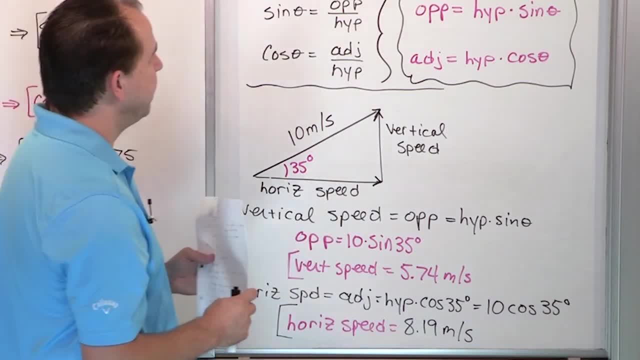 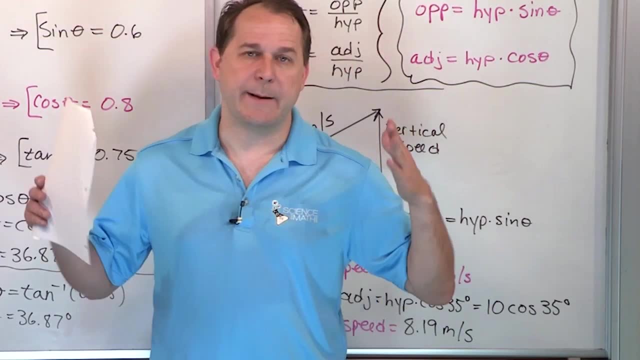 And that's true. So why did I bring this up? Because probably the most important thing in trigonometry that you will learn in physics- and this is why I'm turning around and I'm looking right at you, because I really, really want you to remember this- 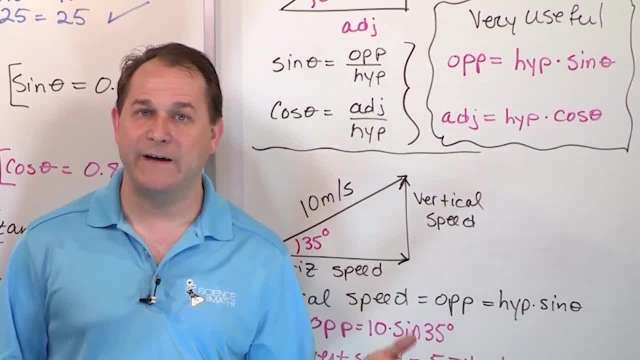 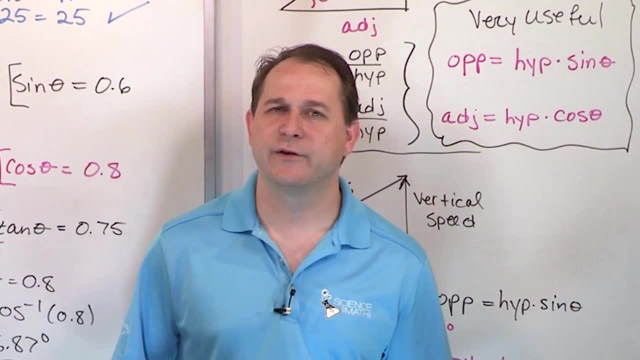 is. we use triangle trigonometry to take what we call vectors and break them up into what we call components. This, 10 meters per second, is called a vector. Please don't let the word scare you. Vector is not a complicated thing. It means I throw a ball at a certain speed. 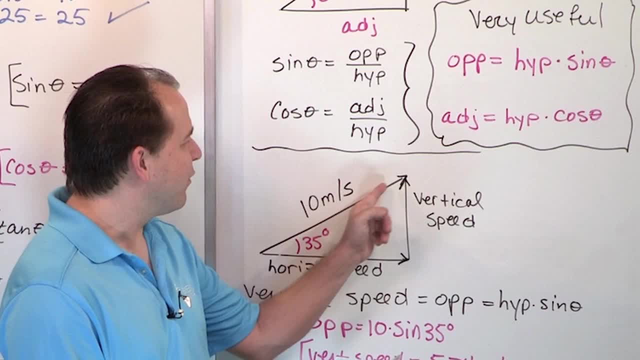 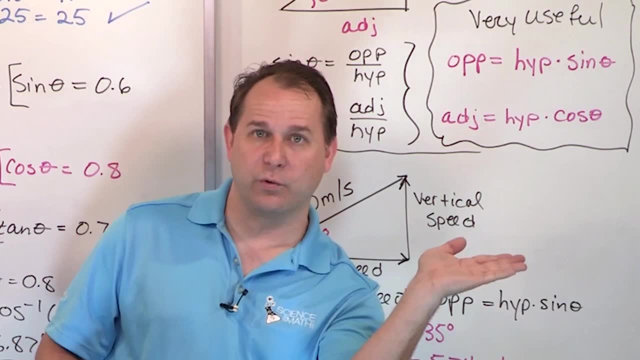 I mean, you know that That's not that hard to know. The length of this arrow is 10, okay, But maybe I don't want to just know what that angled length is. I want to know how much is in this direction: horizontal. 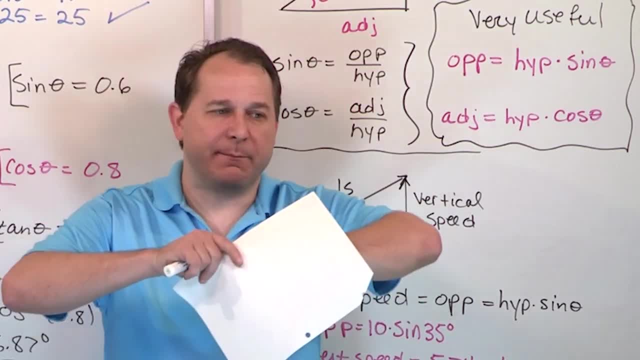 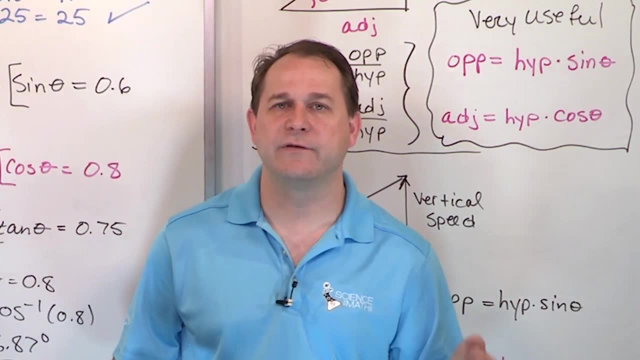 and how much is in this direction vertical. So we take that vector and we break it into components, meaning a horizontal direction and a vertical direction, And we use sine cosine tangent every single time to do that, mostly sine and cosine to do that. okay. 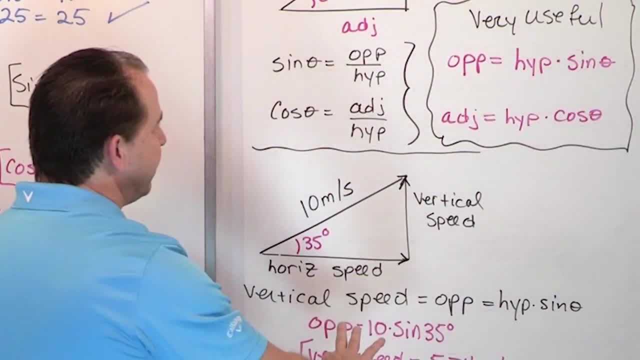 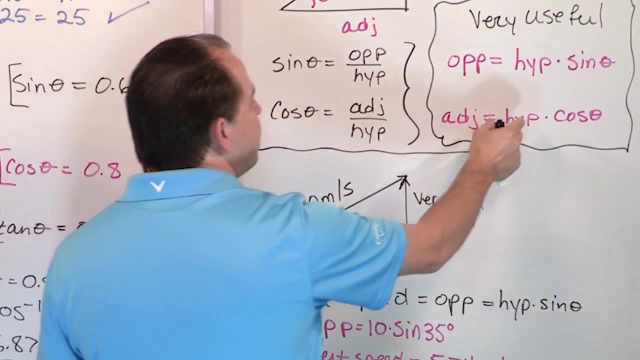 So here's the, Here's the equations that I taught you and then we applied down here. The opposite side of a triangle is hypotenuse times sine. The adjacent side of the triangle here is hypotenuse times cosine. Hypotenuse is the total speed in this example. 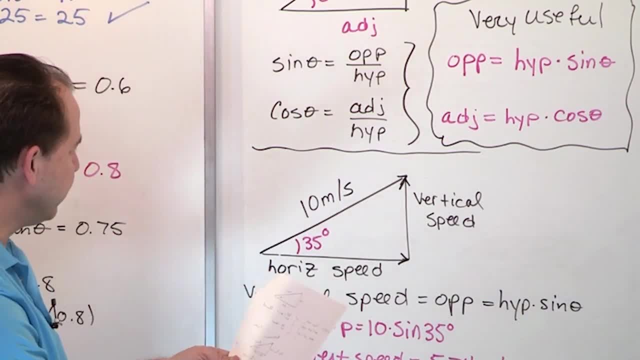 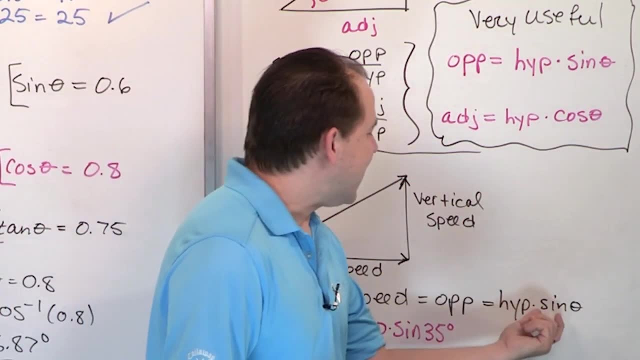 10 meters per second that I've thrown the baseball. Here's what I have written in my notes. I'm not going to write it down, I'm just going to say it about four times to make sure you understand When we use a sine function. 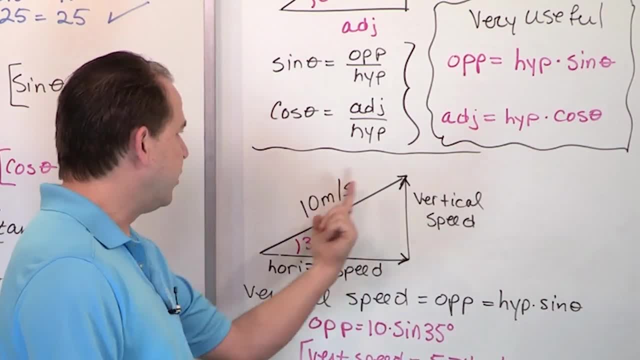 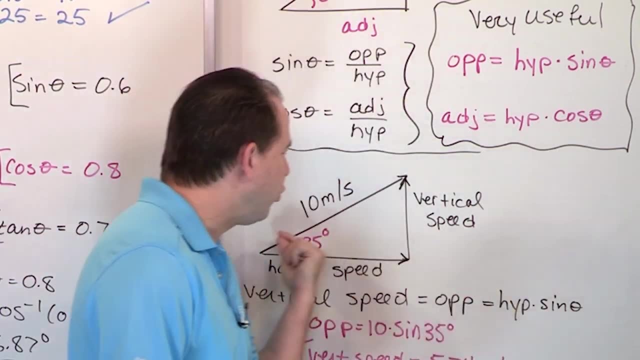 and multiply it by the total length of the baseball speed. okay, In this case, what the sine is doing- listen to me here- is it's taking the total speed 10 meters per second and it's chopping. it is what I have. 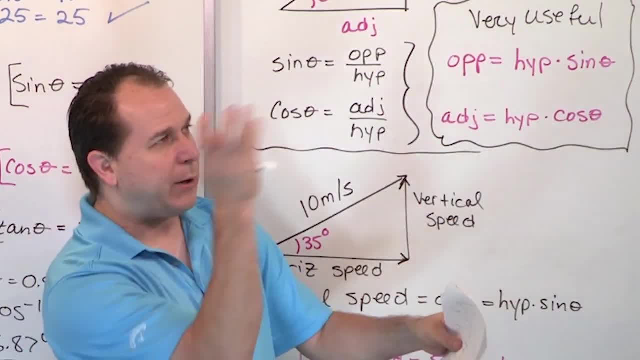 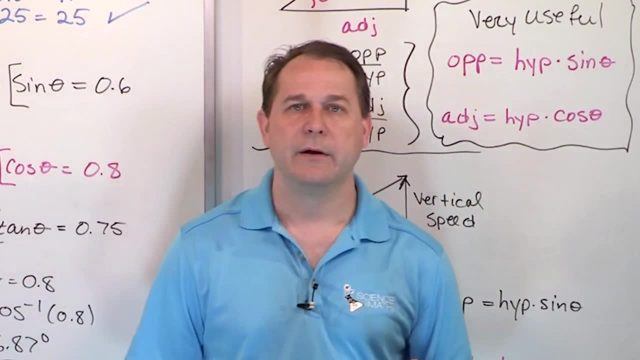 Actually, this is the way I think about it. It's chopping it down. You throw the ball at 10 meters per second. but I want to chop it and I want to know only how much is going in the vertical direction, That's, the opposite side going up. 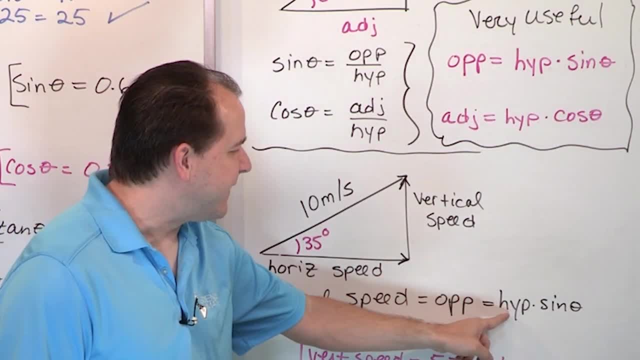 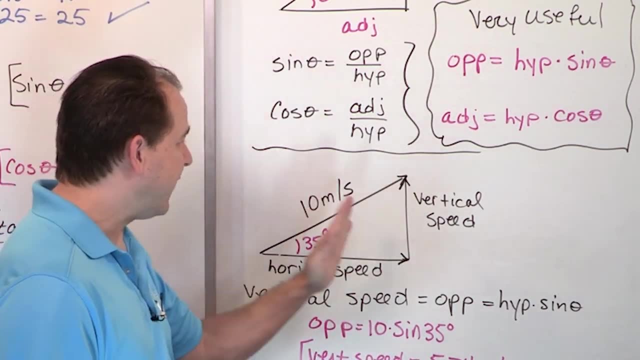 So when you take a sine of an angle and multiply it by the hypotenuse, what you're doing is you're taking the total speed and you're chopping it, finding how much of it goes In the vertical direction, because vertical is opposite. 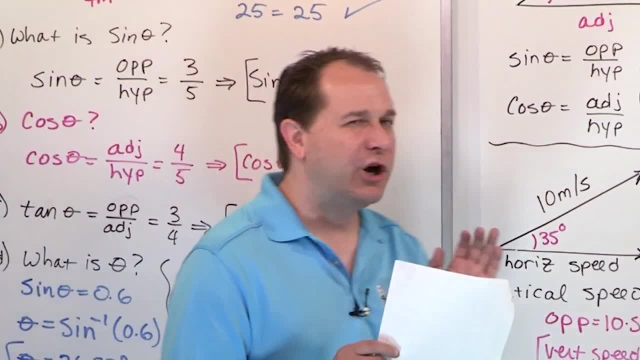 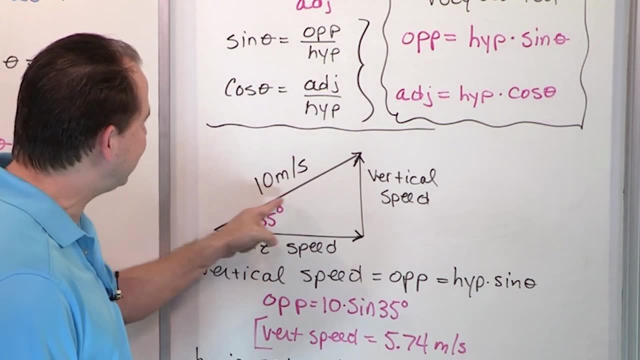 Remember I told you, sine always deals with opposites and cosines always deal with adjacents. And that's to help you remember that when you take the sine of this angle and multiply it by this, it takes this number and it chops it. 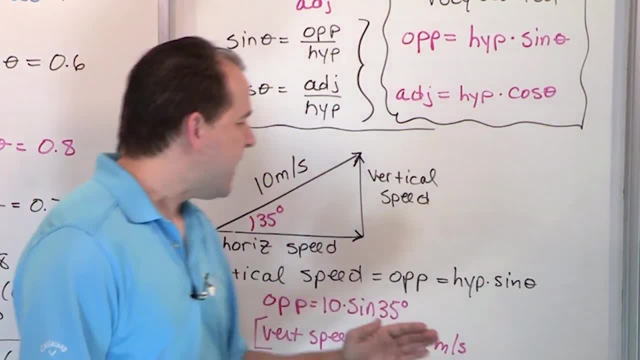 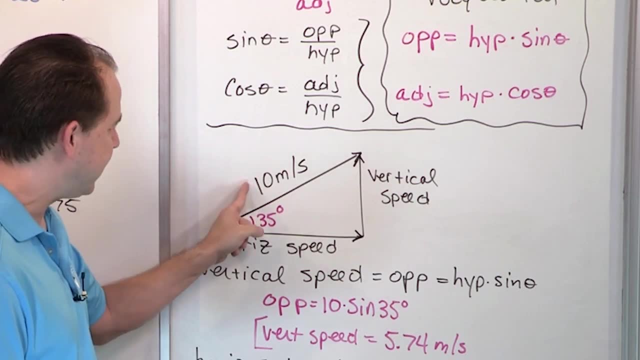 only to give you the vertical part of the speed right. And when you take this number and take its cosine that deals with adjacent. So when you take the cosine of this and multiply it by the same thing, you're chopping it also, but only getting the horizontal part. 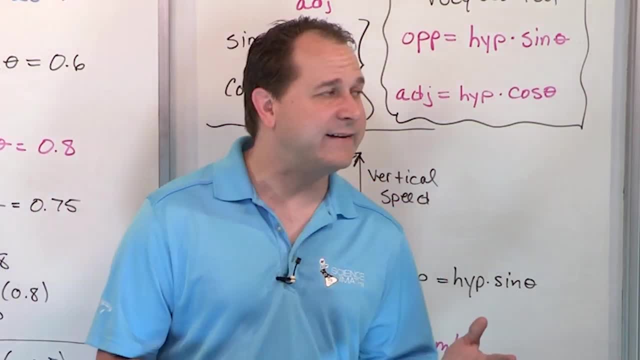 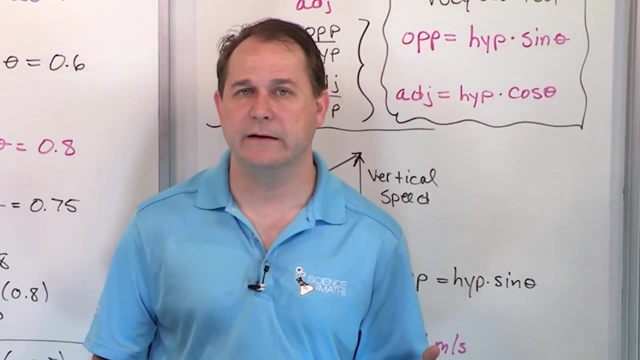 which is this. So here's the moral of the story, because in this case I've given you a speed at 10 meters per second at an angle, But this vector thing we haven't talked much about. it can represent lots of things. 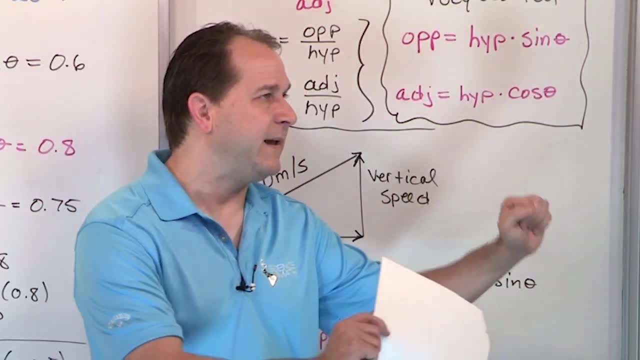 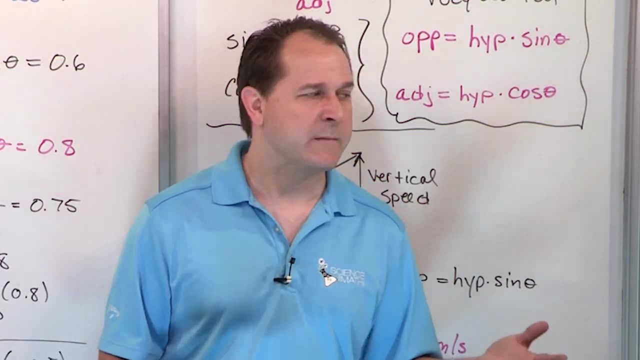 It can represent a force. Maybe I'm pushing on something at an angle and I'm pushing with 100 pounds of force or 100 newtons of force. We'll talk about newtons later. It's the unit of force, okay, But I want to know not how much am I pushing at an angle? 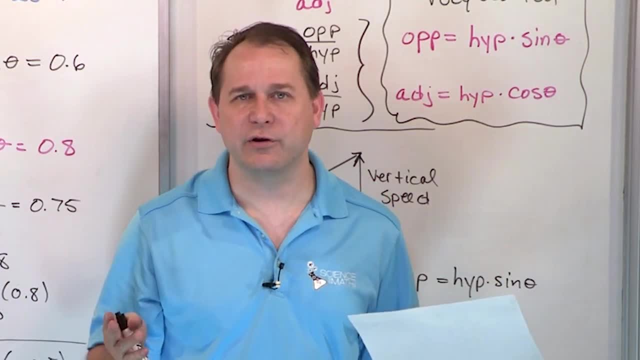 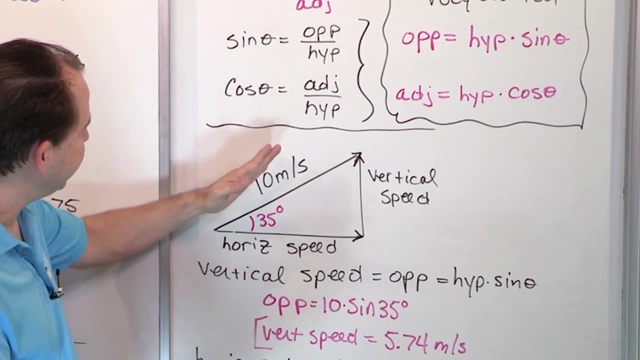 how much am I pushing horizontally and how much am I pushing vertically? Well, I do that by using a vector. I take this. when I multiply it by the cosine of this, it chops it and gives me only the horizontal part. When I take this and I multiply it by the sine of this, 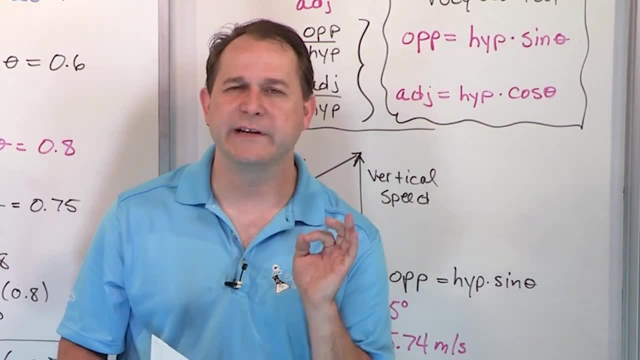 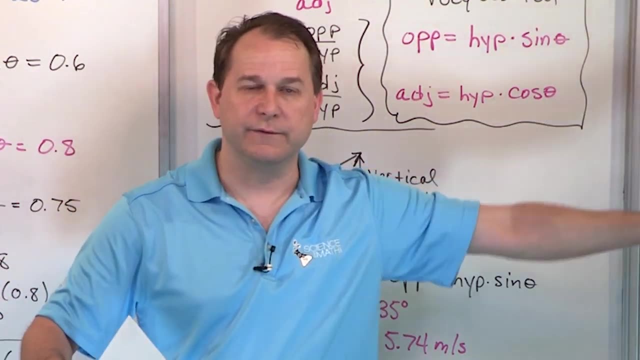 it chops it and it only gives me the vertical. It's crucially important because all these physics problems, what we're going to do, we're going to break them all apart into x-direction and we're going to solve those, And then we're going to break them separately into y-direction. 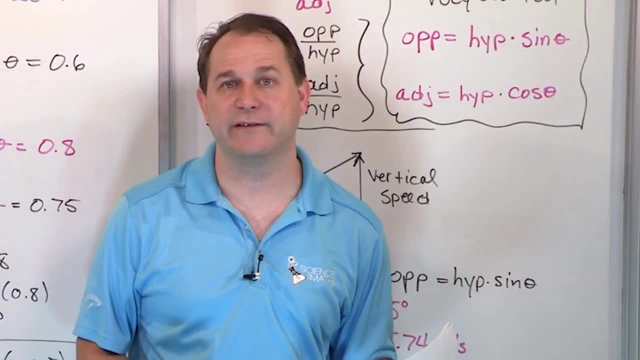 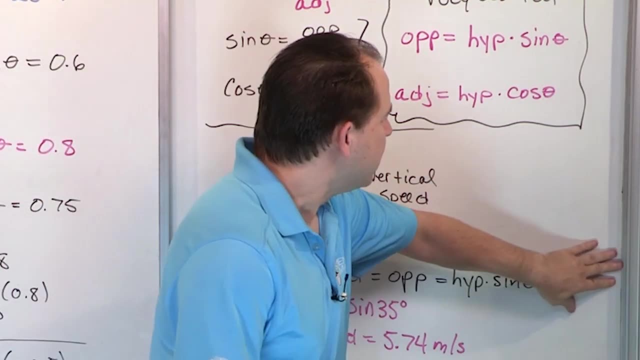 and we're going to solve those. We're going to break everything apart and solve the different directions separately. It's important to be able to take this and chop it this way and chop it this way to get the two different components. So here is your mega, mega, mega summary. 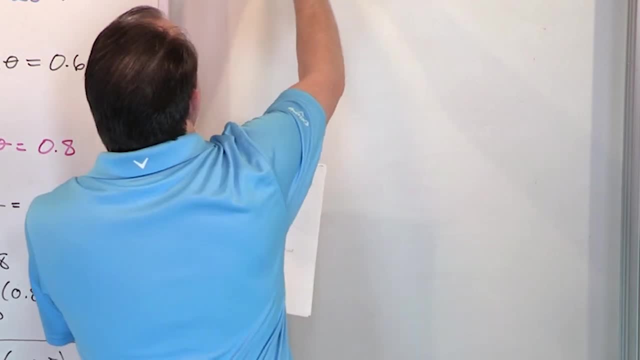 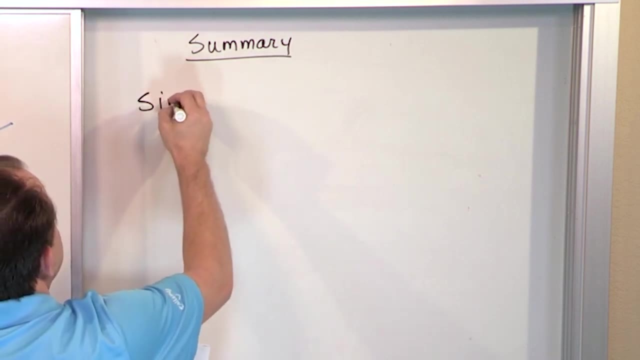 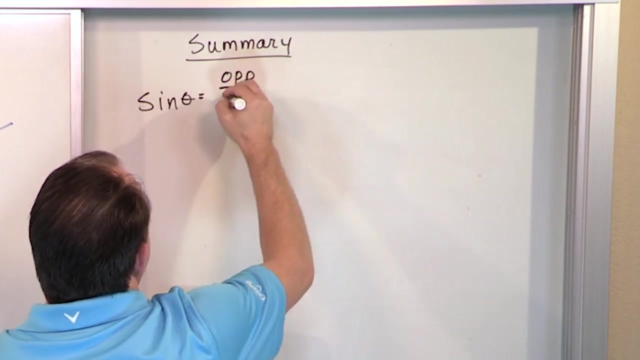 of everything we learned in this section. Summary summary. all right, Here's the summary. When we have a triangle like that, the sine of an angle is the opposite. whoops, the opposite over the hypotenuse. the cosine of an angle is the adjacent. 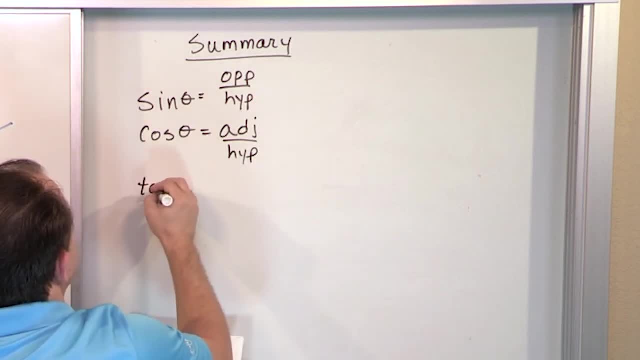 over the hypotenuse. The tangent of an angle is the opposite over the adjacent, so it doesn't involve a hypotenuse there. okay, Now we can take these guys and we can find, use these equations to find the angles in every one of these cases. 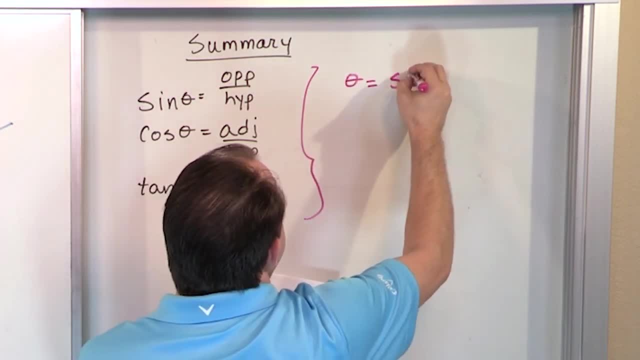 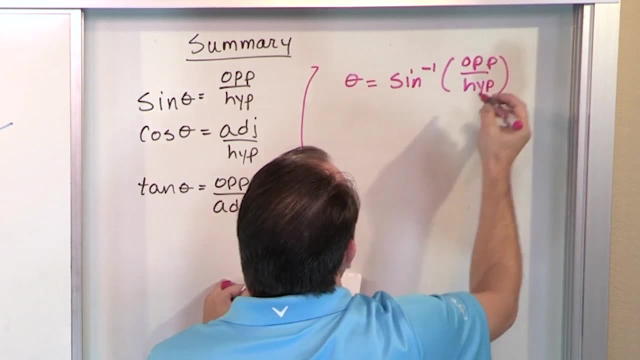 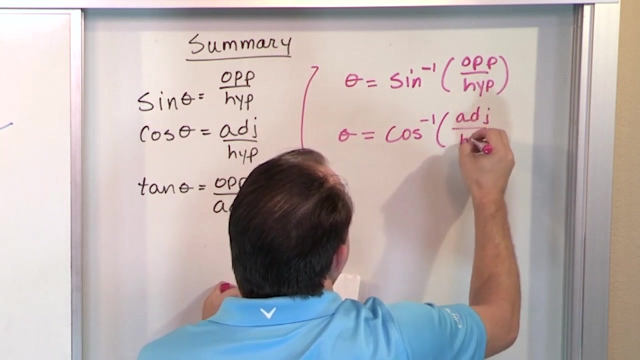 How do we do it? We can say that the angle is equal to the inverse sine of the exact same thing, opposite over hypotenuse. We can say that the angle is also equal to the inverse cosine of the adjacent over the hypotenuse. 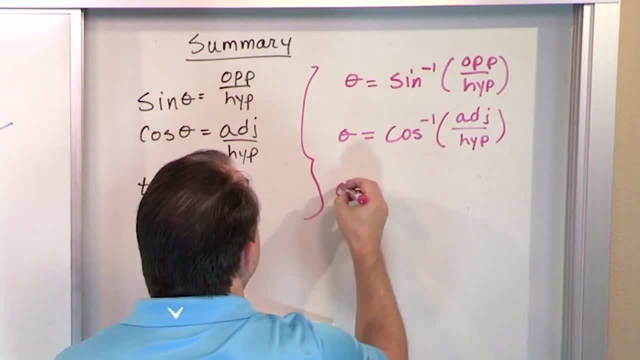 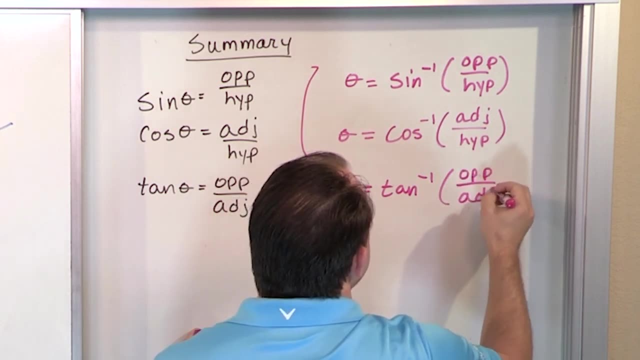 And we did an example showing exactly that. And we can say that this angle is also equal to the inverse tangent of opposite over adjacent. Literally, you take the fraction, stick it in there. If you want to find the angle, you just inverse it. 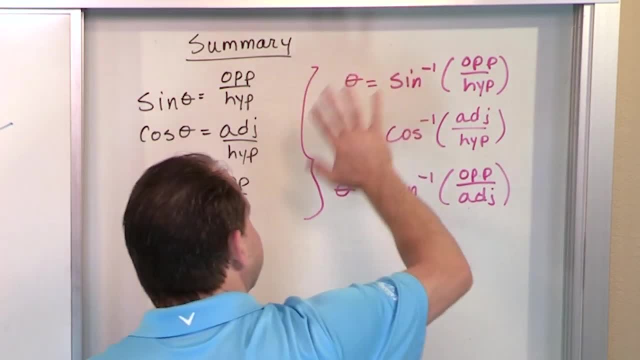 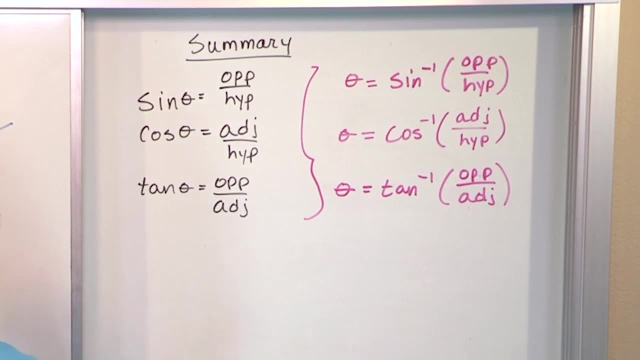 That's all you do. okay, Which one of these is correct? They're all correct. You can find the angle using any one of these relations, and we actually showed you that A minute ago. And then the final thing I want to point out is that we can take these equations: 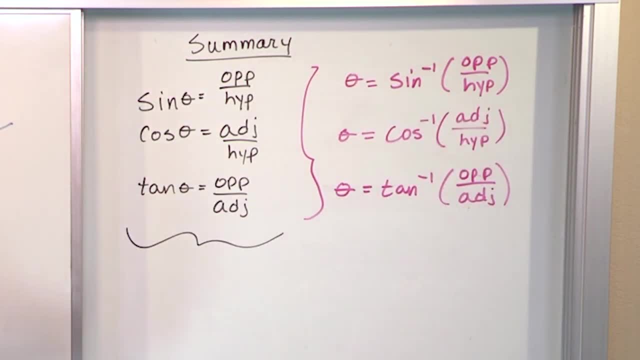 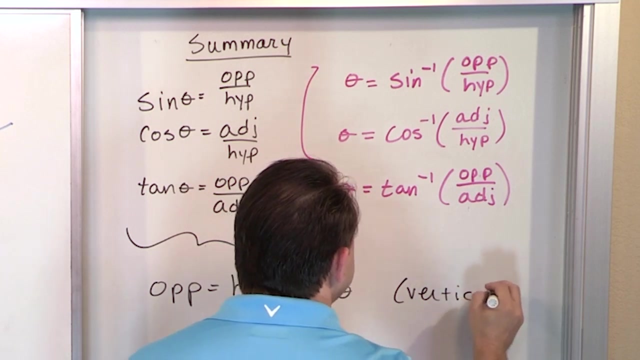 so that's a useful set of relations. We can take these set of equations and we can write even more useful set of relations. We can say that the opposite side of a triangle is just the hypotenuse times, the sine of the angle That's going to give you the vertical, if you kind of think of your triangle the way we've been drawing it. 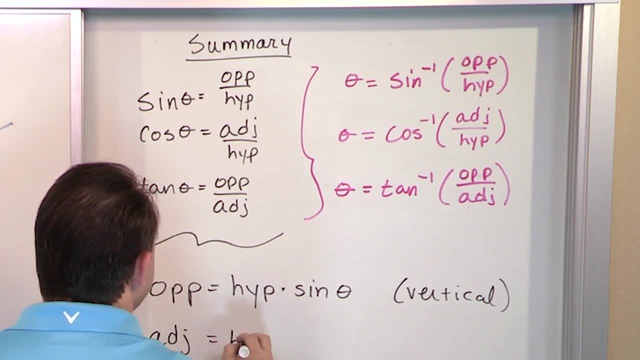 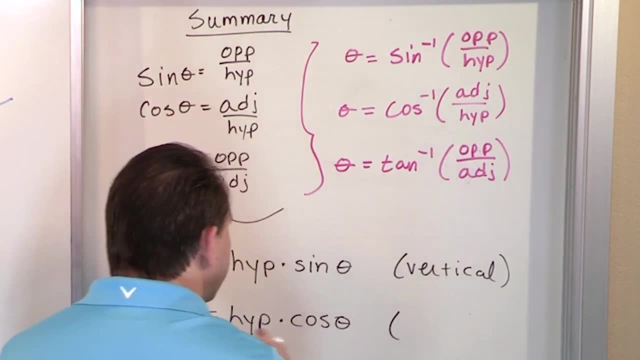 And the adjacent side of that triangle is the hypotenuse. It's the hypotenuse times the cosine of the angle. The sine chops this thing to give you the vertical part, and the cosine chops this thing because you're multiplying by the hypotenuse. 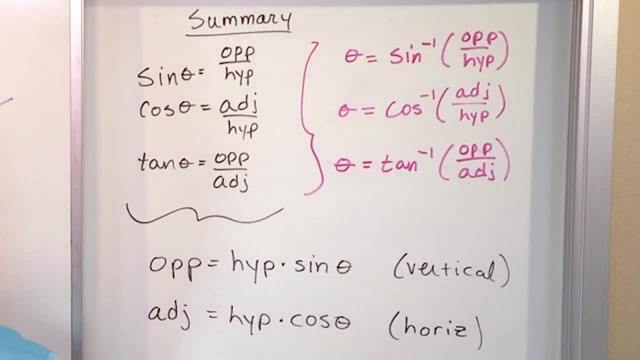 giving you the horizontal part. So when you look at a trig book or a physics book, you'll see these equations, you'll see these equations and you'll see these equations and it gets very confusing. Which ones do I remember? Really, all you really need to remember are these. 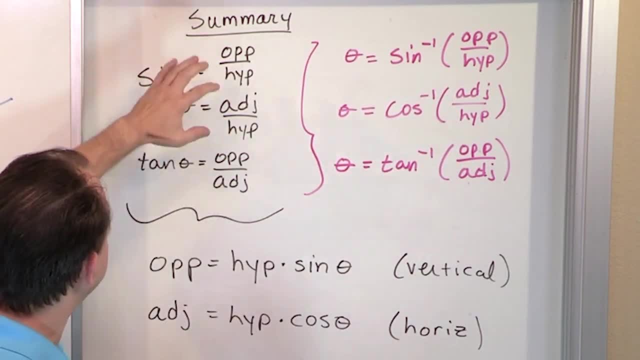 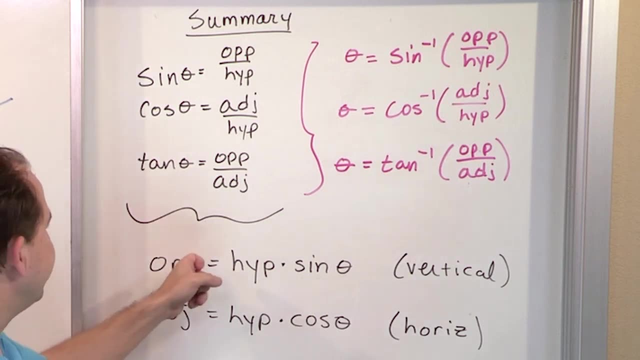 These are the core equations. These just come from these. These just come from these. So, really, just remember these. But what's going to happen is you're going to use these so much that you will remember them To find the vertical part of a vector. 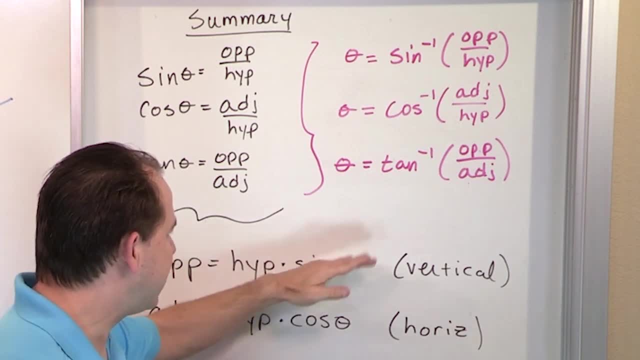 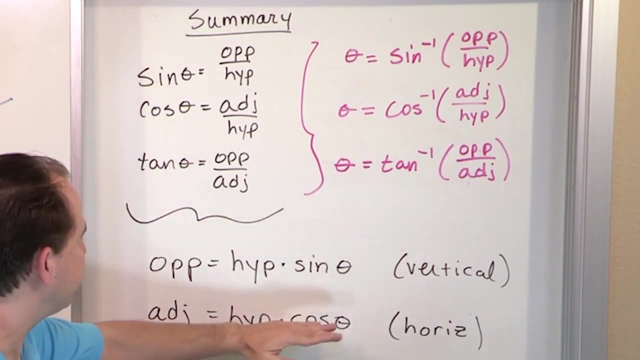 you're going to take the hypotenuse and chop it with a sine. Chopping with a sine gives you that vertical part To find the horizontal part of some vector, some arrow, some hypotenuse of a triangle. you're going to take the hypotenuse and you're going to chop it with the cosine. 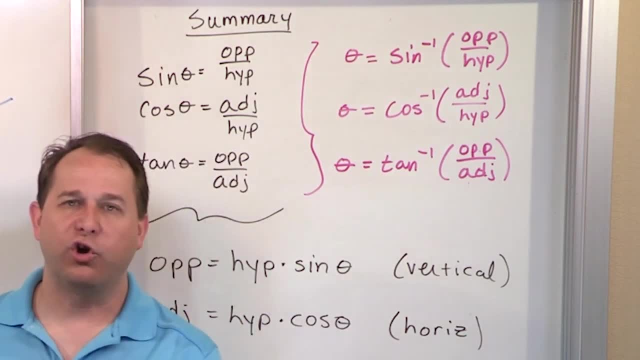 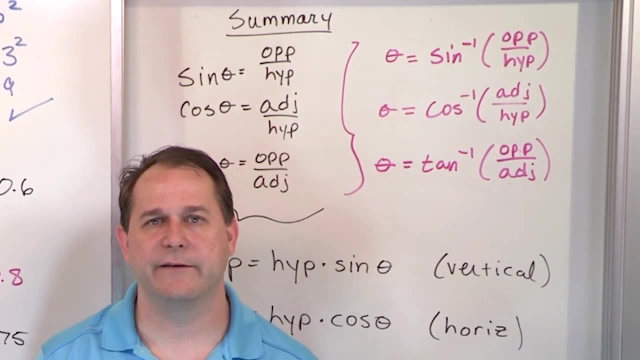 That gives you the adjacent or the horizontal part. Those are the core things of trig. When you take a trig course you'll do so much more than what we've done here. You will plot sine cosine And you'll see that sine and cosine go up and down like waves. 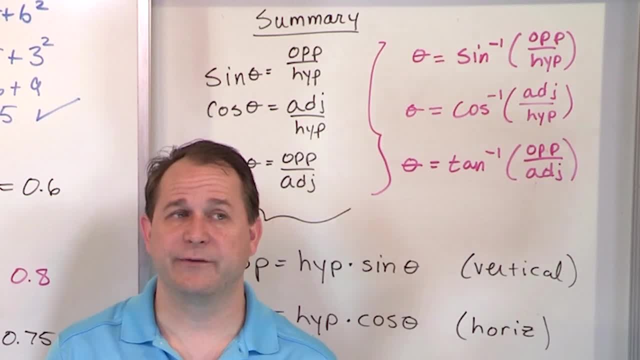 And you'll see that tangent looks even crazier. And there are other trig functions besides sine cosine and tangent that you'll learn in a trig course. In a trig course you'll also learn- or a precalculus course, you'll learn about the unit circle. 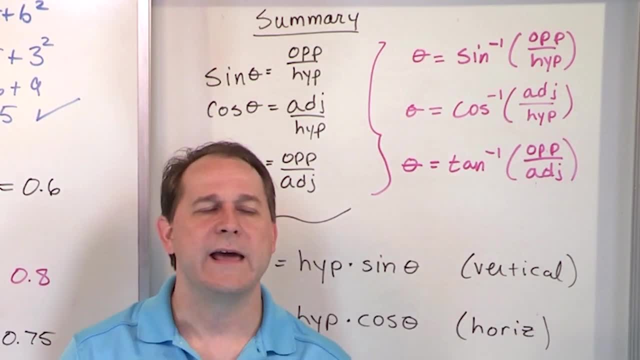 And you'll learn about how to calculate sine, cosine and tangent using the unit circle. And you'll learn about radians And you'll learn how to convert radian measure to degrees, because that's a unit of measure of angle also. But in physics, which is what I'm focusing on, these are the most important things. 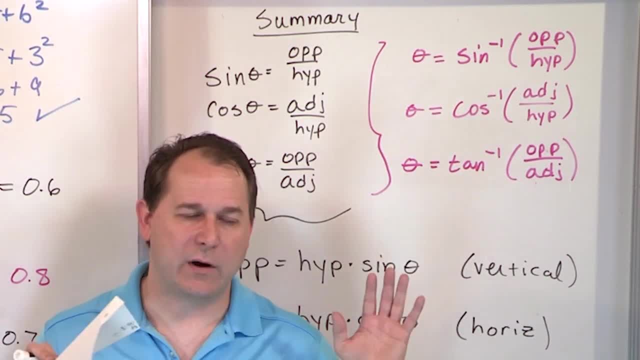 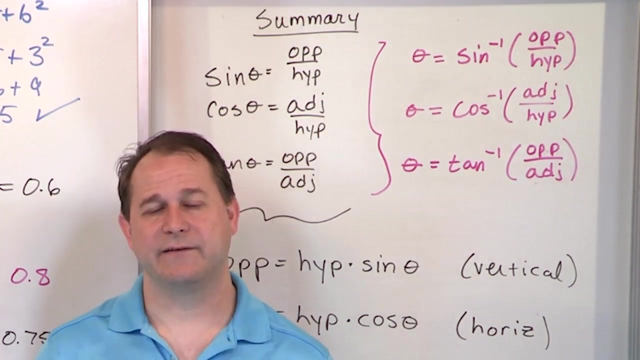 These things are important. If you don't understand this, watch it a few times. If you don't understand anything about it, then go review trig using my trig and precalculus class And then come back here and continue learning physics with me, where we'll do everything step by step and give you plenty of practice to do really well and get a deep understanding of the topics.